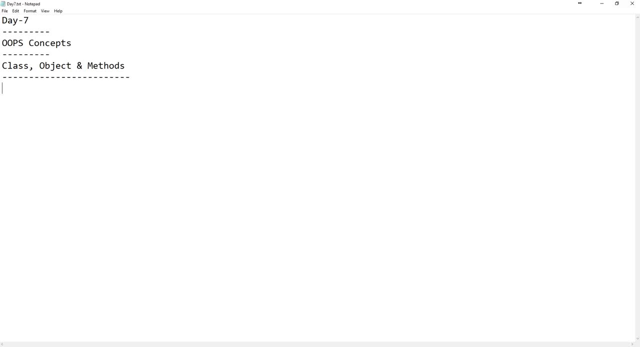 object-oriented programming languages And visual basic, C, and these languages comes under the structural programming languages, whereas C++, Java, NET- So these are all languages- comes under the object-oriented programming concepts. So today we will understand. So for what we? 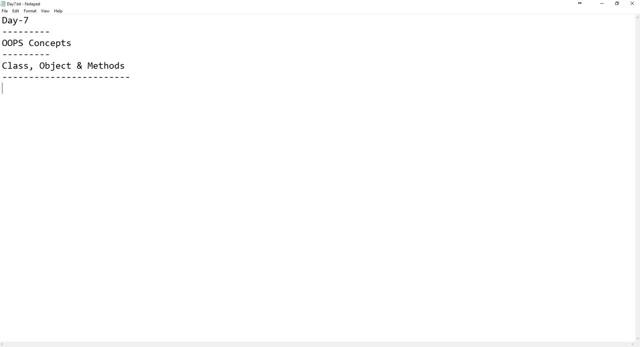 have covered is a basic programming concept, So like data types, operators, arrays, string methods, So these are all will be available for every programming language, But especially the OOPS concepts are available only for object-oriented programming languages. Now, when I, if I want to write a simple program in Java, we have to create a class. 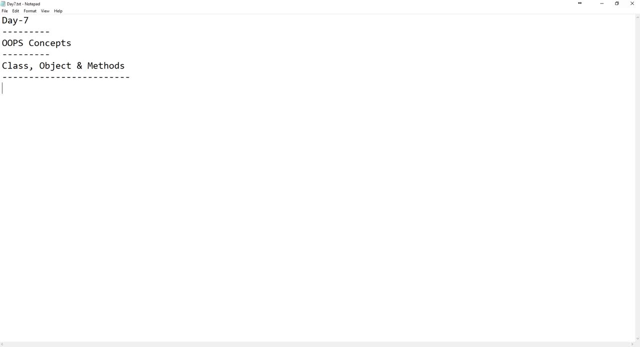 right. Without class we cannot even write a single line of the code in Java. So Java is an object-oriented programming language. Why we are calling Java object-oriented oriented programming language? because the programming, the java, will support certain concepts, so those concepts are called as object oriented programming, concepts like classes. 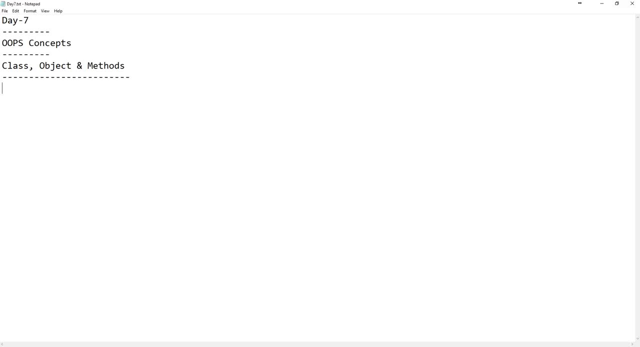 objects, inheritance, polymorphism. okay, so these are all the different concepts which are comes under the object oriented programming. so today we are starting about few concepts under oops: object oriented programming, class, object and methods. so far we are using class because when i want to write a small program, we are creating the class and also we have used object, but we 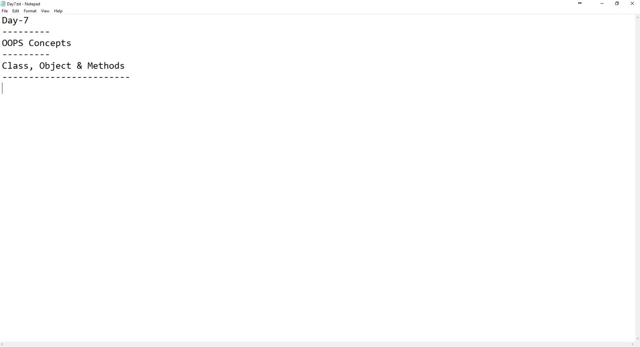 don't know exactly what is class and what is object. also we have used methods, but we don't know exactly what it is internally, how it will work. but indirectly we are still using classes, objects and methods. the terminology we know, but what is exactly? class- object oriented programming. class- object oriented programming. class- object oriented programming. 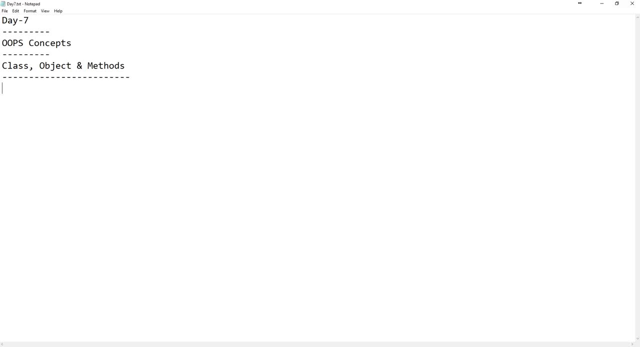 object, methods and what is the importance of that, how object oriented programming will work. so let us understand with some example: class, object and methods. what is class, how to define a class and what is an object, why we need to create an object and what are all methods. let 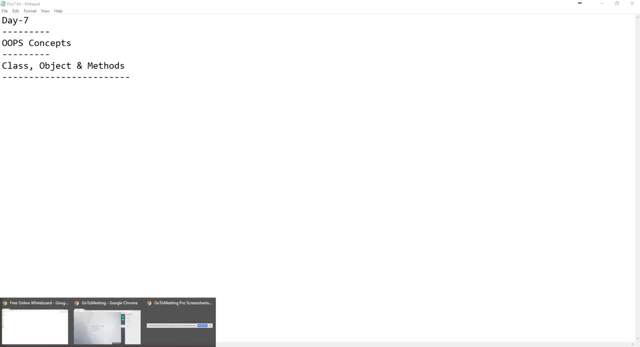 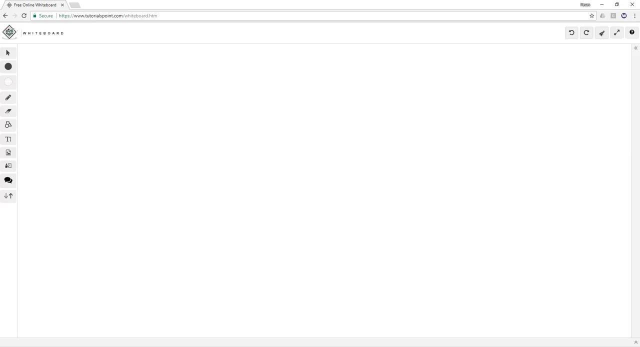 us discuss that part. so first example: if you see the real time example, in real world everything is an object. what we can see is called as object, even a human or animal, a bird, everything is an object. whatever we can see physically, that is an object. so for example, if i say, when i say human beings, right, so human beings means there are number of. 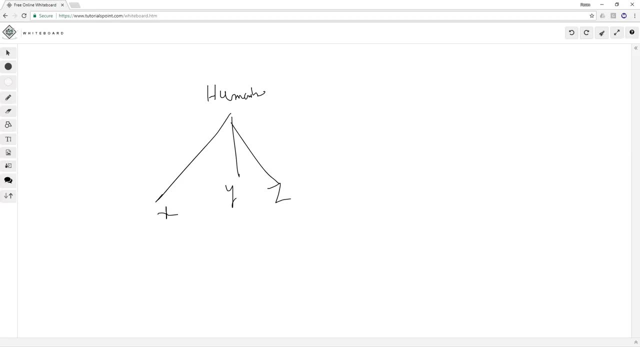 people, some x person or y person and z person. these are all the names of the persons, right? so these are all comes under one category based on certain properties, but they are common properties and we are called them as a human being. similarly, there are some creatures who are having the same common properties. 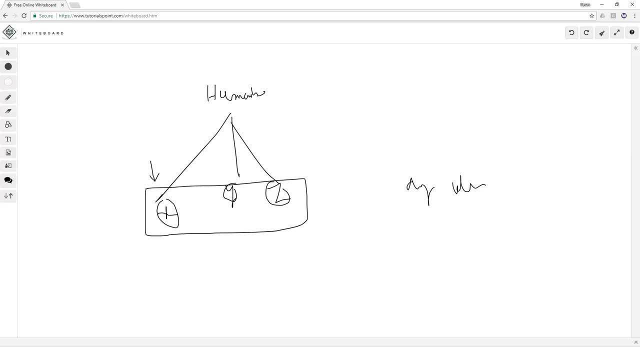 like dogs or elephants or cats. these are all different kinds of animals we are calling as animals, but these creatures having a common property, so that we can categorize and put together, we can call as a animals, right? so, if you observe these two examples, so these are the physical object, physical object which we can see and feel. 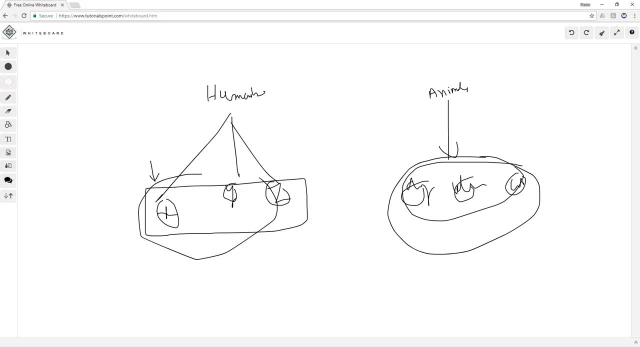 and they are having some properties, some behavior. but when you come here these are all abstract because that we cannot see. animal is a class, basically one category that we cannot see, but all these animals are comes under one category, that is animal category, because they are having the same kind of behavior or properties or color, somehow. 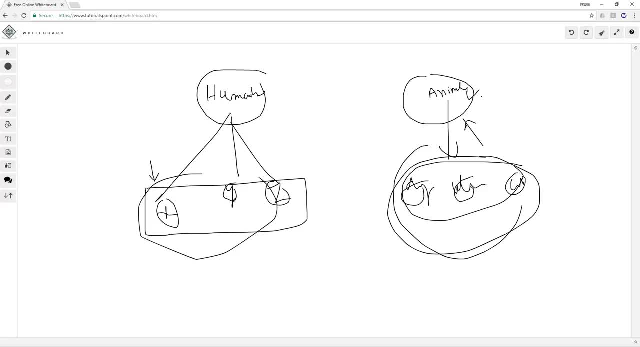 but all are put under one category. that is the reason we are calling as animals, same thing applicable for humans. and similarly we have some vehicles under. vehicles may have two wheelers, four wheelers and so on. so all these things are having some common properties, so that we are comes under one. 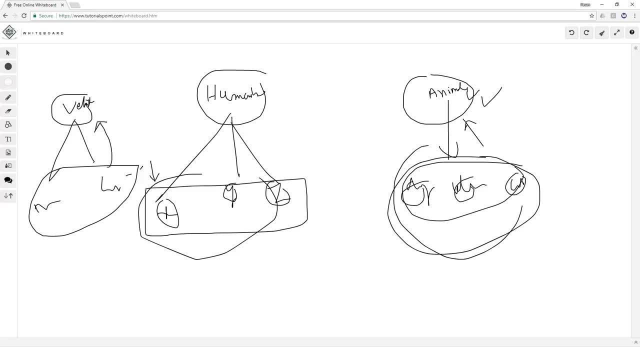 category come, that is, vehicles. so, if you observe these examples, what are all we can see? there comes under the objects, and whatever we are cannot see, there comes under the classes. okay, so a class is a, the logical entity is a physicist. so the class is a logical entity, whereas an object is a physical. 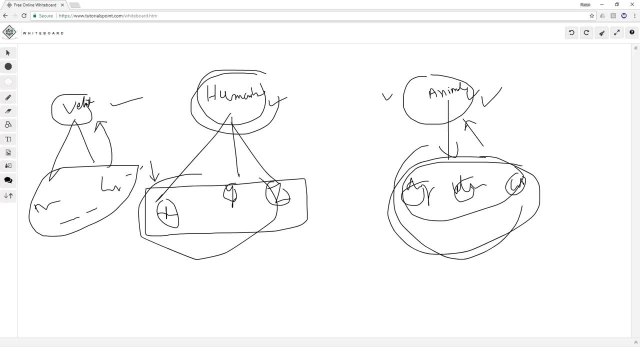 entity. so class is a logical entity, whereas an object is a physical entity. so how we need to define the object, so java is also followed. the same concept, so technically. so these things we call as a classes, animal or human beings or vehicles. these are called as classes. 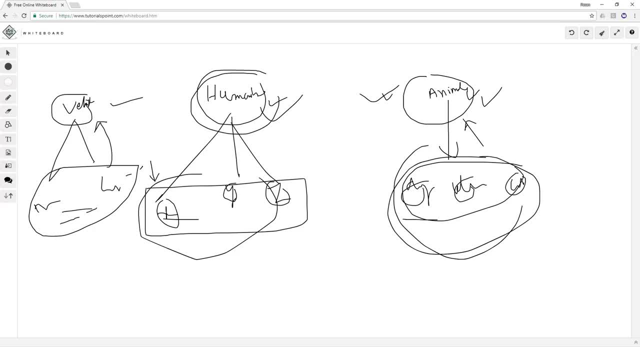 are called as objects simply say so. a class is a logical entity, whereas an object is a physical entity. there's a one definition. the other definition is: an object is an instance of a class. an object is an instance of a class. so when i say some object, you can simply say what is a class for? 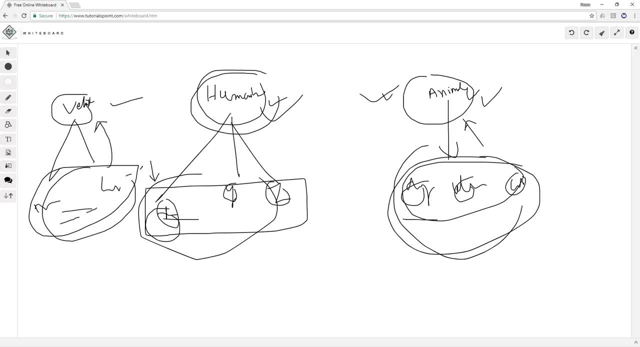 that okay. if you say some person name, you can easily say he's a human being, right? so in that way we can also categorize. similarly like based upon the object right, object properties or common properties, we can say certain class name. so object is an instance of a class. so if you want to create 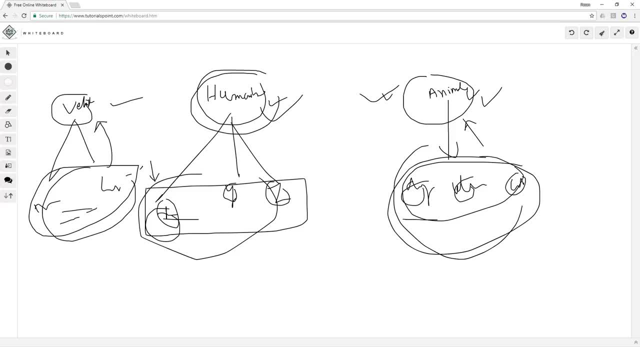 an object class is required. if i don't have class, we cannot create object. okay, that is one thing. so other point is we can just define the class, we can just declare the class in java. we cannot use the class directly. if we want to access the information which is there in that class, we have to create an object. 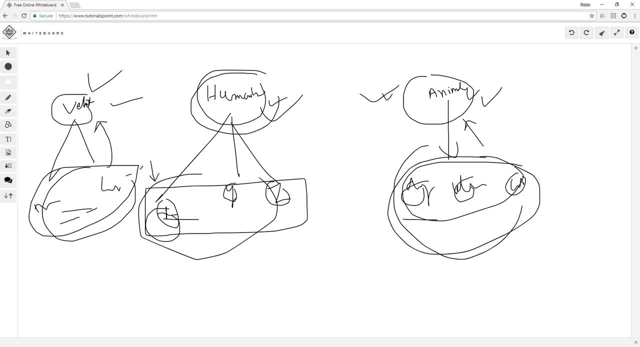 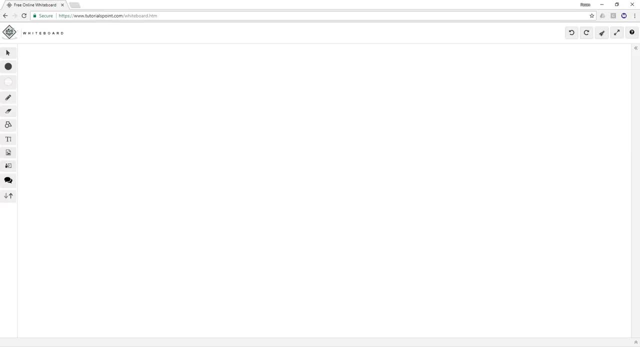 through object we can access. so let us see one more example where class and object will come into the picture. if i say one organization, any organization, there are n number of employees working now. all employees are having certain common property, like every employee is having employee name, employee id, designation, salary right department. 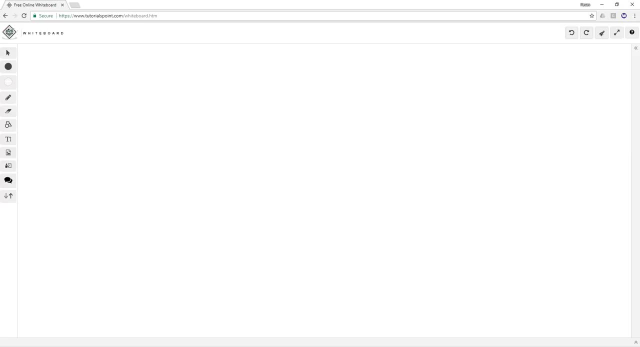 so different fields will be there, but overall all employees are belongs to one category, that is, employee category. right, so now, if i define a class called this is a class, let us say this is a class. the class name is, let us say, employee, this is my class name and this class contains certain. 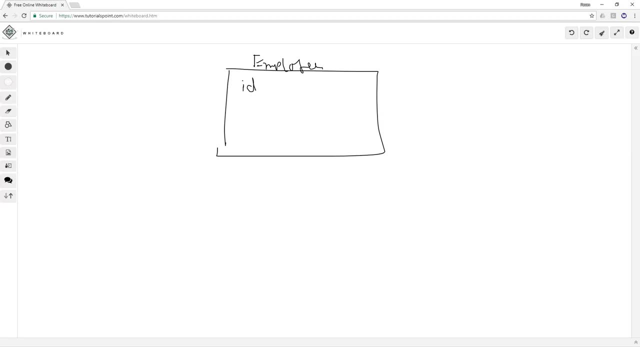 variables like employee id. every employee is having some id. ids can be different, but everyone is having some id. every employee is having some name. every employee is having some designation and some department number, right and salary. so these are all the common things which every employee is having. 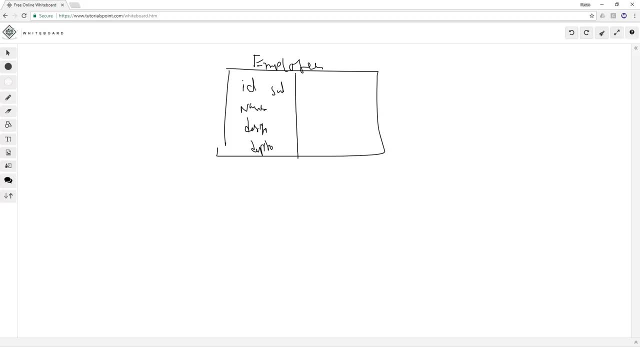 and if employees are getting some bonus. right, if i define one method here, let us say one method here, this method can be applicable for every employee. okay, joining or relieving, suppose. if i define two methods- joining method and relieving- so these two methods can be applied for every employee. so this is basically the class now. based upon this class, we 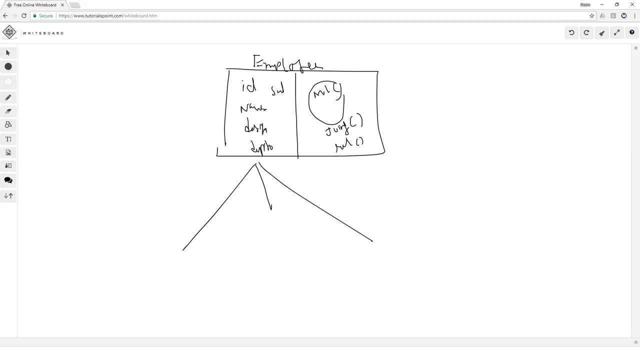 can define n number of objects, like: suppose there is x person joined in company, so this method will applicable and this employee is also having id name, designation, department number. but these employees having its own values, and if i say some x person came and joined, he is also having its own values, his own id name. 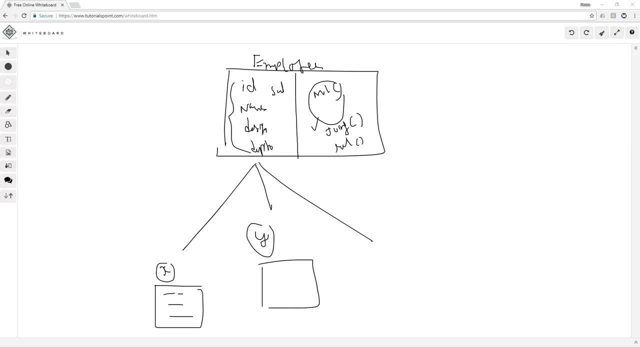 designation, department number, and similarly the other person is also same, having the same thing, one second right. so other employee, let us say jet person, he is also having the same properties like id name, designation and department number and the same methods. so we can define any number of objects like this for the same class. so if you want to define a class or if you 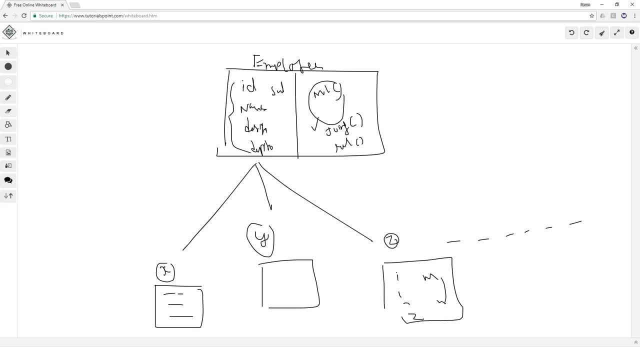 want to derive a class, we have to define class. that's the first thing, and the class, an object, is an instance of the class. if i create an object for a class, this object, everything, will acquire everything from the class. so every object contains id, name, designation, department number and every. 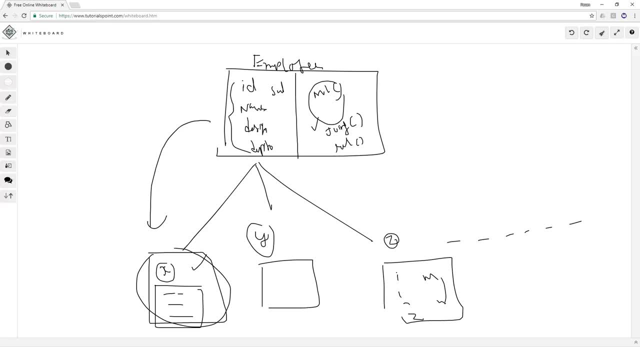 object will occupy the object, name, designation, department number, and every object will occupy the the memory. so this memory is different and this object memory is different. this object memory is different, but the class doesn't occupy any memory because this is a logical object. so all objects are physical object. these are objects which 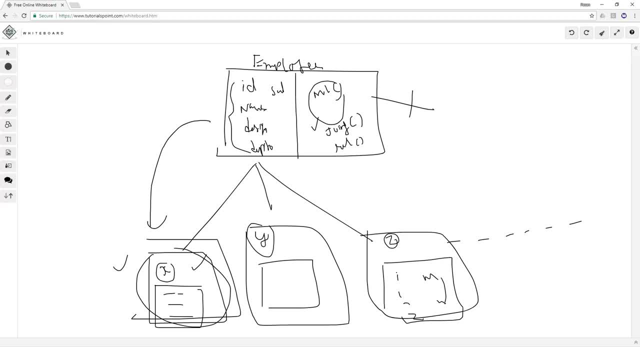 we have created are physical because they will occupy the memory. even though the objects are sharing this information, common details, the memory is different, so there is no such relation between these objects. there is no relation between these objects. but all objects are belongs to the employee, not even two. 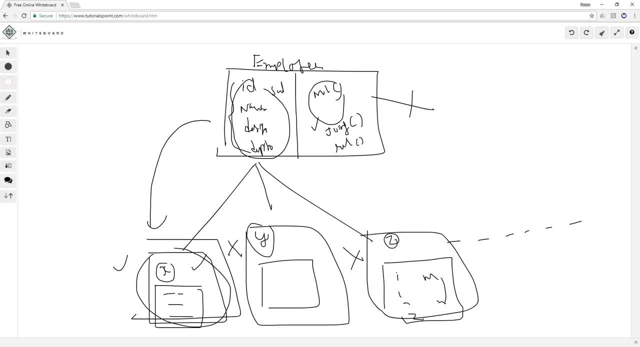 persons in or not even two employees are not same in the organization, but two employees are belongs to the same class, that is employee class. okay, but if you observe the relation between these object, there is no way related these objects, even though they are having the common entities like ID name. 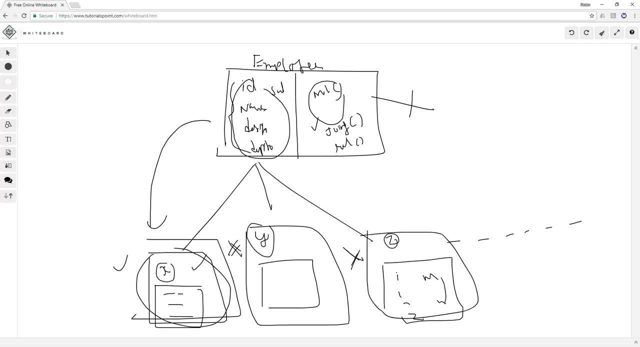 designation. so the name ID, designation, Department, number of employee X is different, then why as well the name is different, z. so this is how. this is a basic concept behind the class and object. now in java, we can create a class if you want to access these variables and if you want to access these methods, we required an 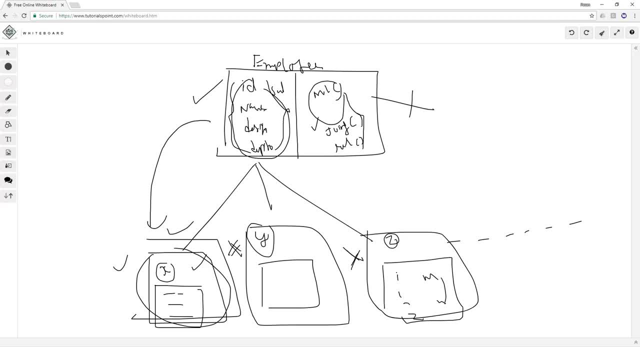 object through object. we can access these variables and methods when i create an object for this particular class. every object is having its own values, like x is having id, name, designation, department number, and similarly y is having its own details. z is also having its own details, but creation of object is same for the same class. okay, now in java, how to create the class. 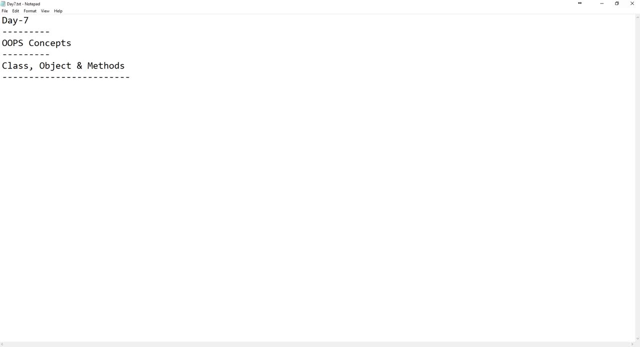 as i said, what is a class? a class is collection of variables and methods. this is the definition of the class. a class is a collection of variables and methods. it contains a and variables and methods. now, object is an instance of class. okay, this is a physical object. 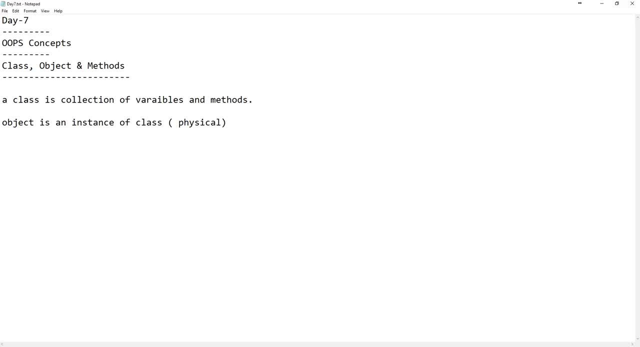 this is a physical. so without class we cannot create an object. and what is method? method is doing some activity within the class. so here, as i said, class is a collection of variables and method. these methods comes under the class. okay, so a method is a method is a piece of code. 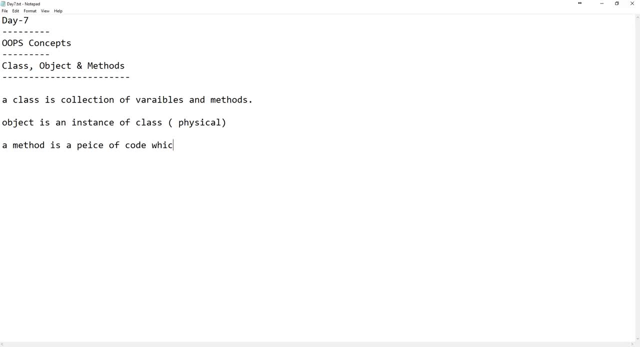 a piece of code which will perform certain task. which will perform certain task. okay, so a class is an instance. a class is a collection of variables and methods. an object is an instance of a class. a method is a piece of code which will perform certain task. all the methods should be part of a class. all methods should be part of a class. 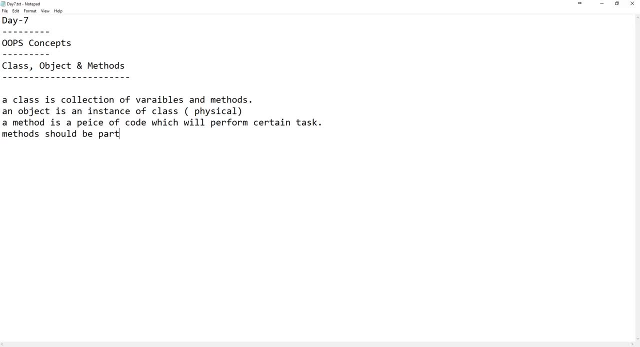 methods should be part of a class. okay, so just remember this point. so now let us see how to create a class. what is the structure of the class in java? so first thing is how to define the class. class is a keyword. this is a declaration of class. class is a keyword. here we need to specify the class name. let us say: employee is a. 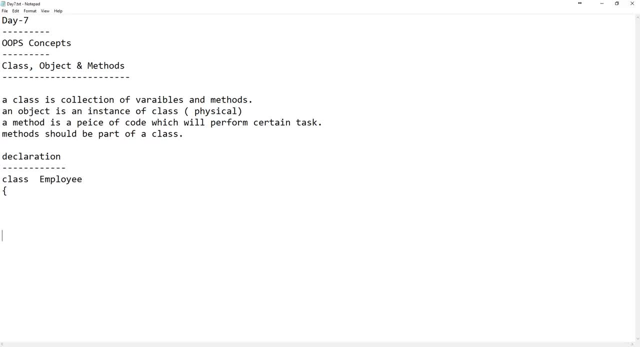 class name and open brace, close base. here we need to specify certain variables and certain methods. so let us say here it contains some variables- variables means employee id name, designation and so on- and also it contains some methods. this is a basic class declaration. now how we can create an? 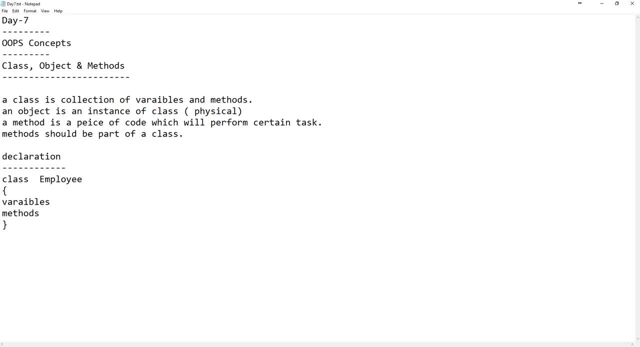 object for this particular class. create an object for the class. so how to create an object for the class. so this is very simple. first class name, that is, employee and object name. let us say emb1, this is my object name, equal to new employee. this is my again class name and brackets and semicolon, so actually the new. 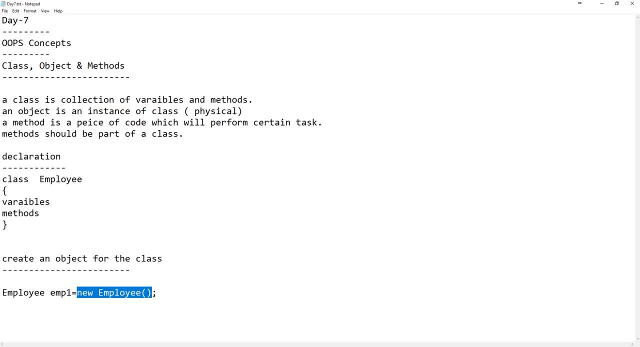 employee we are saying right now is a class name and brackets and semicolon, so this is a class name. so this is the instance of there are three different parts are here. so here employee is the class, employee is a class name, emp1 is a reference variable. reference variable of object and employee. 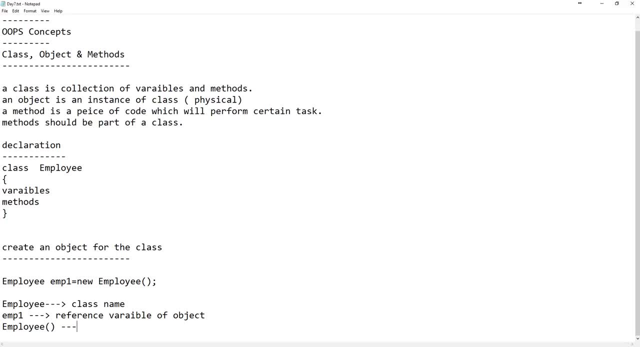 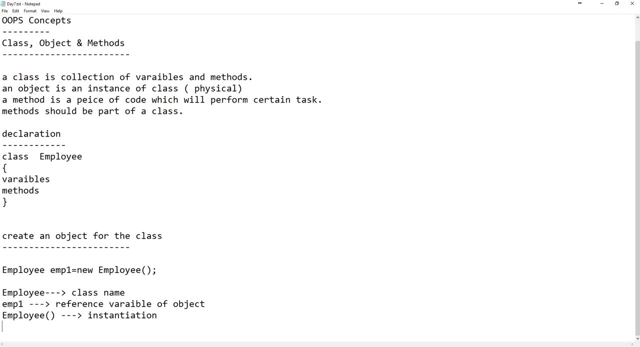 bracket is right called as instantiation instantiation. so without instantiation it not allocate memory to that particular object, so that we need to always instantiate the particular object. so class, employee, object name equal to new, again class name brackets. so this is how we need to create an object now. EMP1 is: 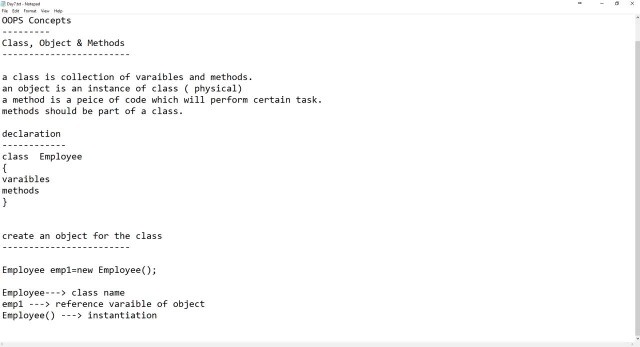 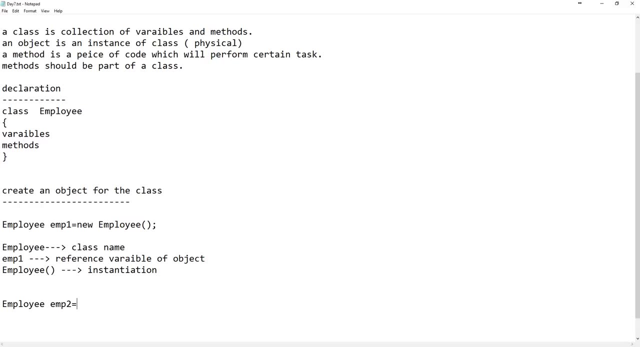 an object. similarly, we can create any number of objects. now let us say I'll create one more object called employee EMP2, equal to new employee. so this is another object. EMP2 is different, EMP1 is different. now all the variables and methods which have declared in the employee class will be. 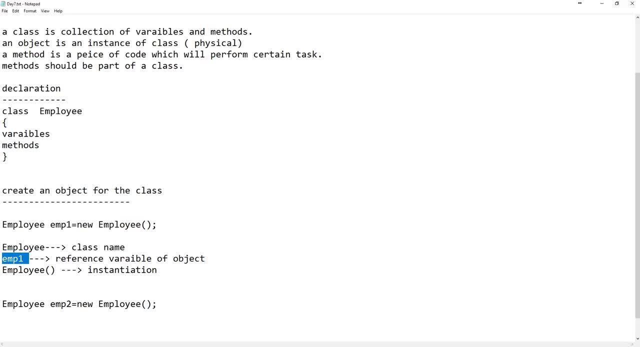 applied for EMP1 as well as EMP2, even though these two employees having the same variables and methods. these two are nowhere related. both are different entities. because both are physical object, they will allocate the different memory locations. okay, now, this is how we need to create an object. now let us see. 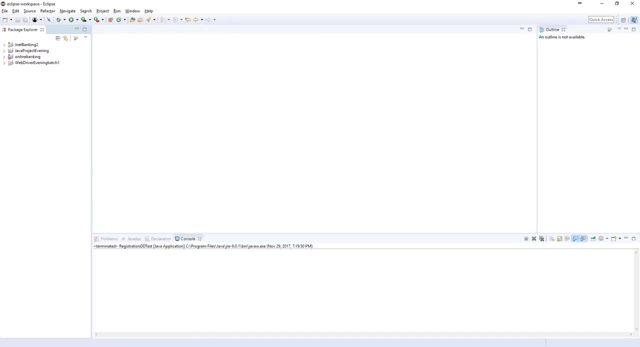 a small example for this class and object. now under Java classes project. here I'll create new package for object oriented programming. so oops, finish. so under this I will create new class called as employee. this is my class name and don't take main method, keep it as is. so now this is a class, so this bracket can be in the next. 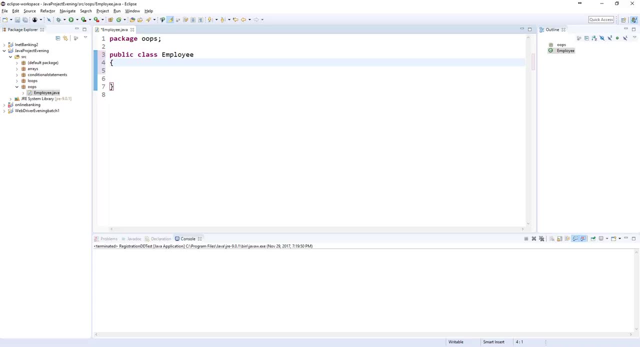 line also not a problem. so this is a class. so this class is present under oops package. there's a reason: at the first line it is displayed as a package: oops. now, inside this particular class, we have to specify some variables and methods, such I said a. 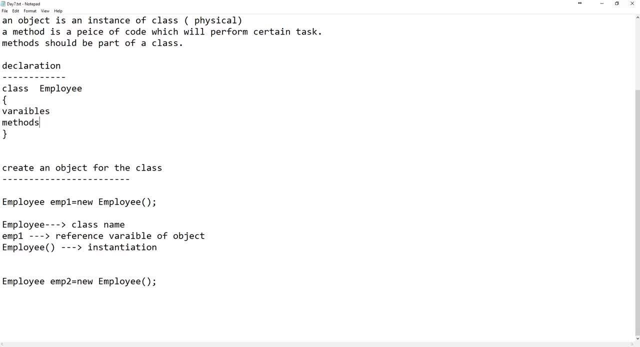 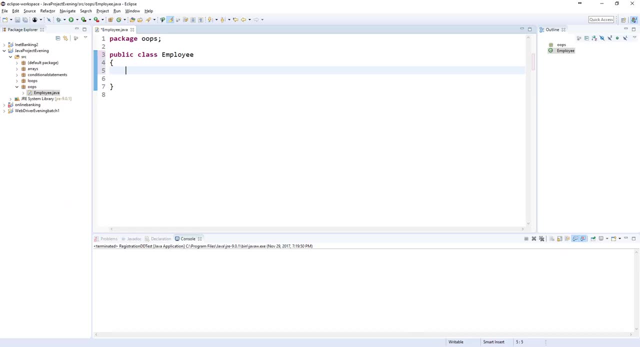 class is a collection of variables and methods. a class is a collection of variables and methods. now, in this employee class, I will define few variables and also few methods. so let us define an integer: is an employer from a class name who is De episodes or variables and methods. whether I define an, 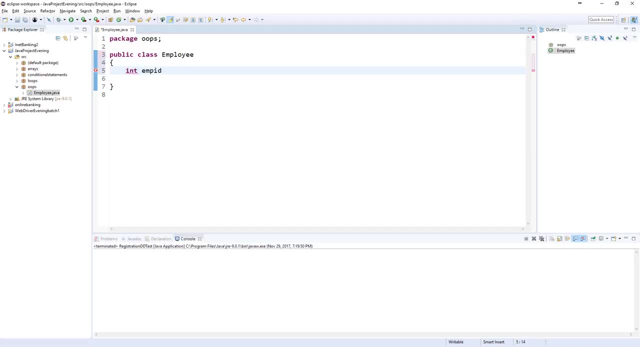 EMP ID. Don't specify any values, because one object to another object the values will be vary. So employee ID and string EMP name. This is our another variable. and let us say integer salary, and I'll say string Department Number, DEPT number. Let us say this: make it as an integer. 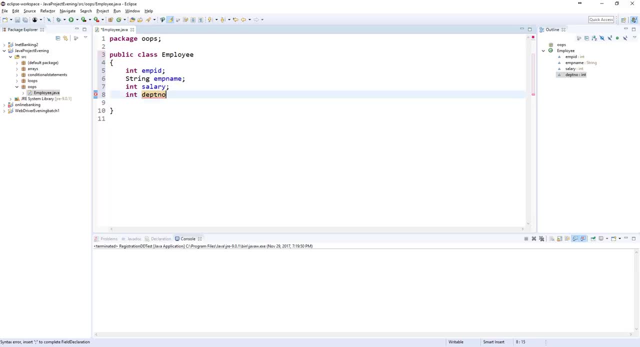 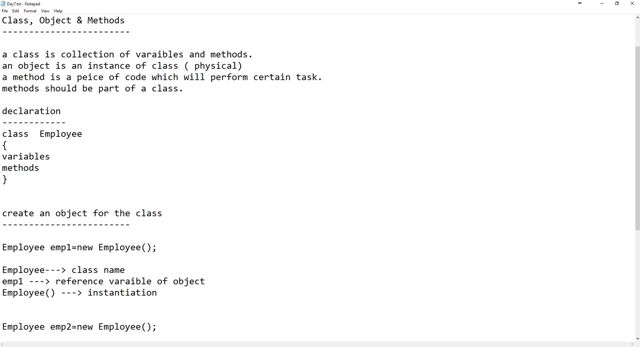 DEPT number, department number, Right. So these are the variables. every employees having these details right. Along with these variables, I will also define few method. So what is method? how we need to define a method? the method definition will be like this: so, syntax of methods, syntax of. 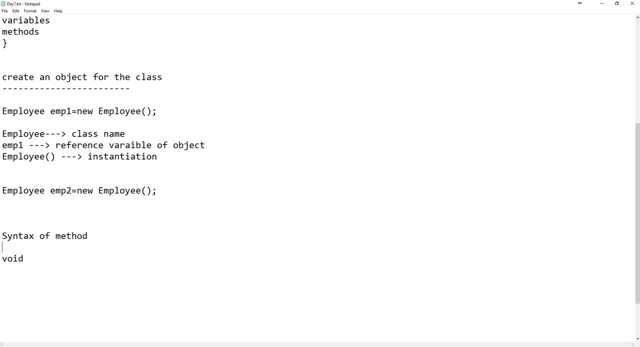 Method. So first we need to start with method name. let us say M1 is a method bracket- Open curly braces and close curly braces. here We can write the some code, Some logic we need to include, and these methods are different types methods. are there some methods? 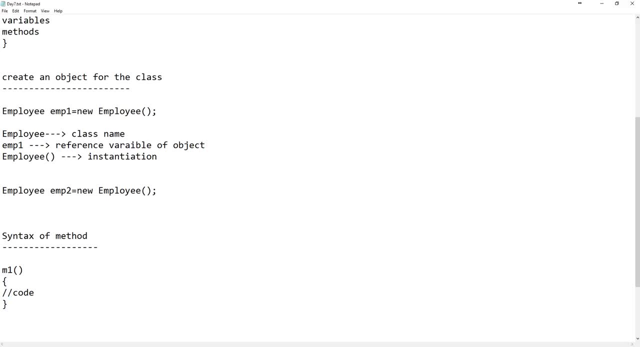 Will return some value. some methods may not return some value. So when I call this method, it will return some value. some methods Will not return any value. So in previous class we have seen some string methods right, So those methods will return some value. always they are called predefined methods which are already there, string method. 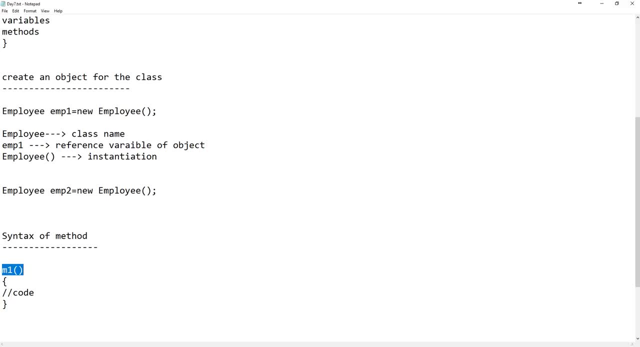 We are just used up use of those methods. but these are all user defined methods. We are creating our own methods within the class. So a method can return some value. sometimes a method may not return any value based upon our logic. Suppose this method is written some value. 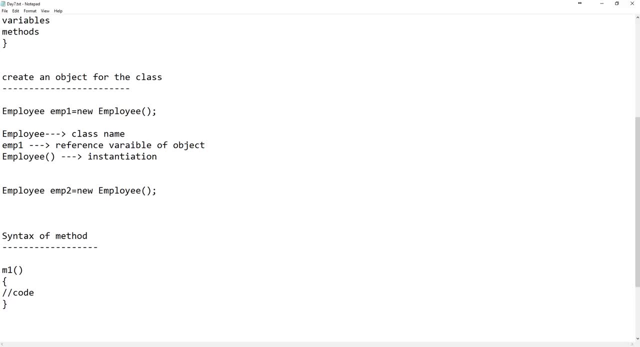 We have to specify the data type or we have to specify the void. Void means this method is not written, anything. suppose if this is returning something, then I need to specify the which data type it is returning and Inside the method also I need to put written statement, written something, some value or integer value. how to return? 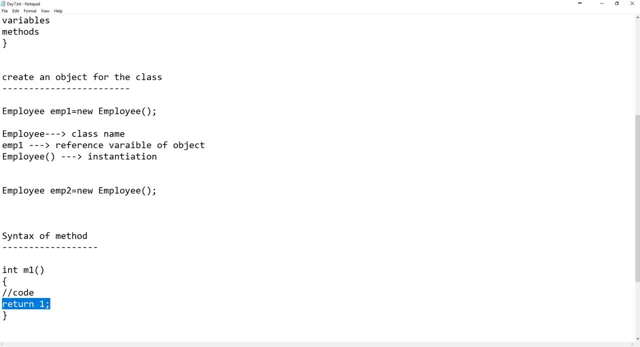 If I have to use this written keyword. before this method You must specify the data type and this one value, and this data should be exact the same. Suppose this method is not returning any value, Just put as a void and this type. it will not return anything. This is a simple method definition. 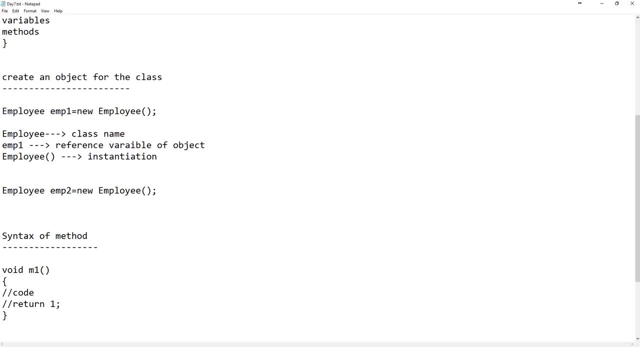 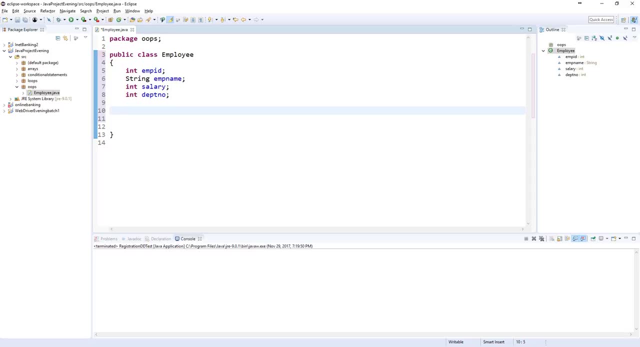 So now in this EMP class, I put some variables. along with these variables, I will also define Few methods. okay, so how to define this few methods? so let me define a method called as Display data, for example, at a 7 display. This is my method. 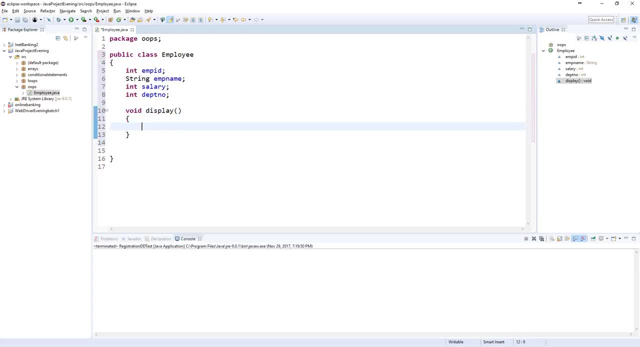 So what this method will do is this method will display all these values: employee ID, name, salary and department. Now here I'll write the code for that, for displaying purpose. So system dot out, dot println. First one is EMP ID, So this I want to print now. second one is: 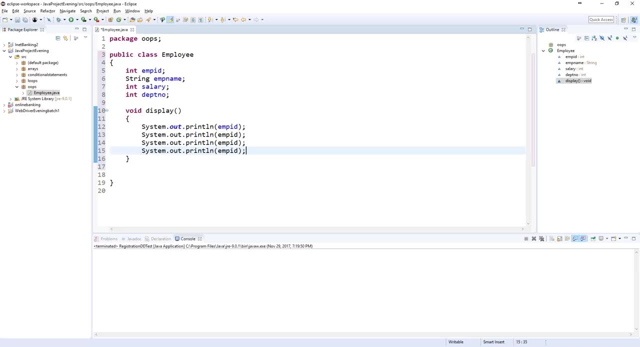 third and fourth. Second one is EMP name and the third one is salary, Then EMP number. Right, so now this is a method I have defined, so it is a class. Class contains some variables and I have different one method. currently I have only one method, okay. 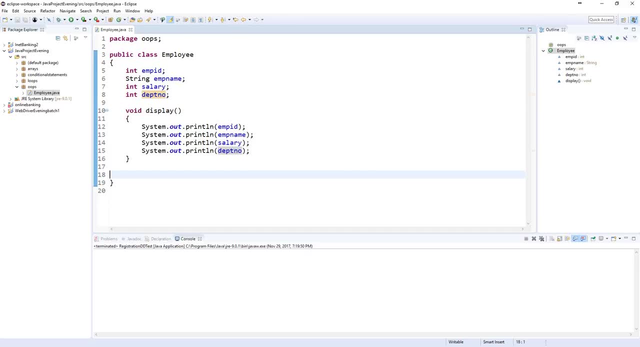 So now this is an entirely we can call as a class. now, if you want to access these variables and this method, We can access through object only. we have to create an object. Okay, so how to create an object so we can create one more method here. 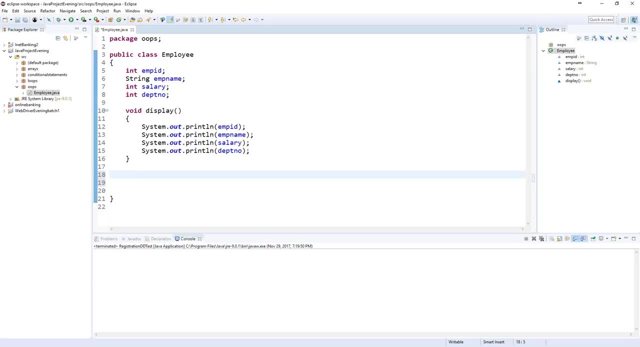 There will be main method, right, because the execution is always start from the main method. So this is a normal method. This is a normal method until unless we call this method, It will not execute. So if you want to initialize these values to those variables, if you want to call this method, 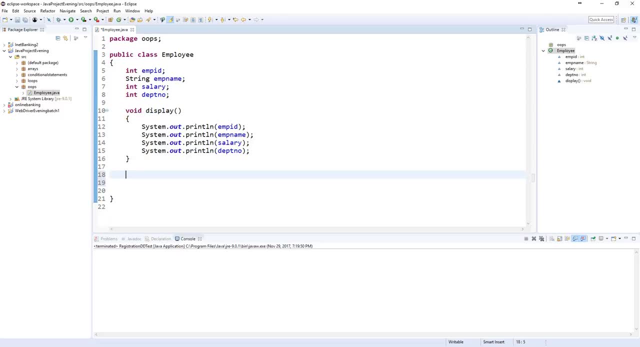 We have to create an object for employee class. So where we need to create an object, We have to create an object always in the main method, because the execution is always start from main. So along with this normal method, now I will create the main method for the syntax of main method. public static void. 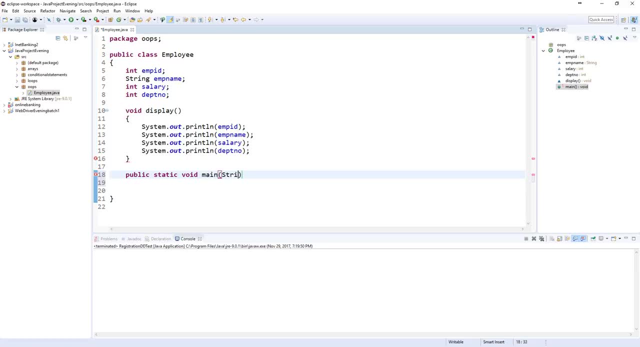 Insert this string arjs. It will take string array as a parameter. Okay, this is a main method now. Now, here we need to create an object and other stuff. This is a main method because execution will start from here, right, so now. So I have to create the object for this particular employee class, right? 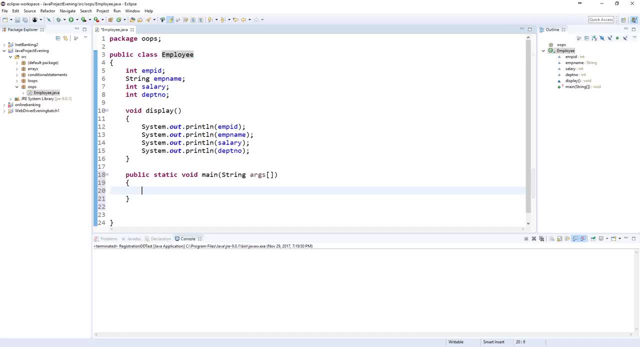 So how to create an object for employee class? as I said, first we need to select the employee class, class name, employee. Let us say EMP1, equal to new employee. So this is an object. EMP1 is referring to employee class. EMP1 is different. now, EMP1 is having all these details: employee ID is having employee name, salary department, everything is having. Now I will assign those values for EMP1. 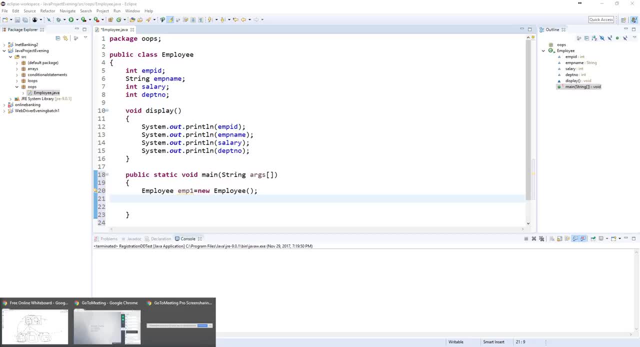 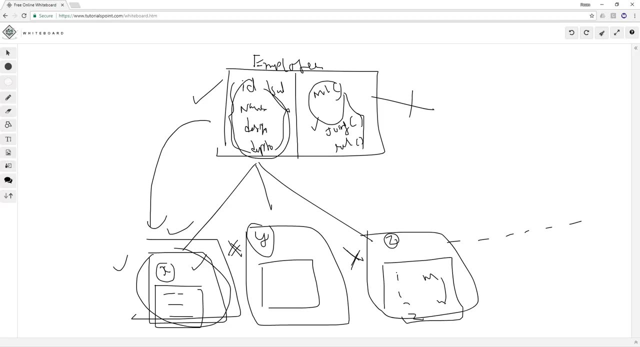 So now, if you see the context here again, When I created some employee here, EMP1- EMP1 ID is different than EMP2 ID and EMP3 ID, So every employee is having its own employee IDs, its own names, designations and department number. 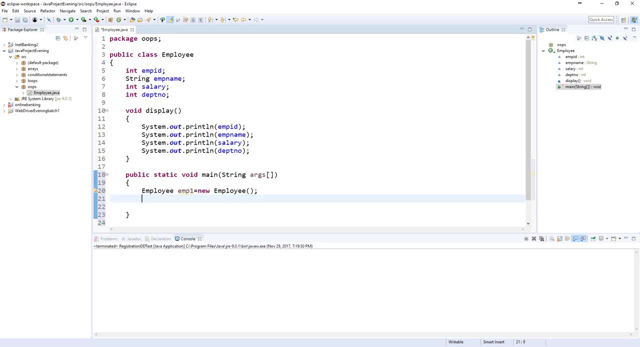 So here I have created an object for EMP1, so now these variables and method can be applied for EMP1.. Through this object I can access this. So now how we can access EMP1.. See, now it is showing all the variables: DPT number, ID, name and signup right. 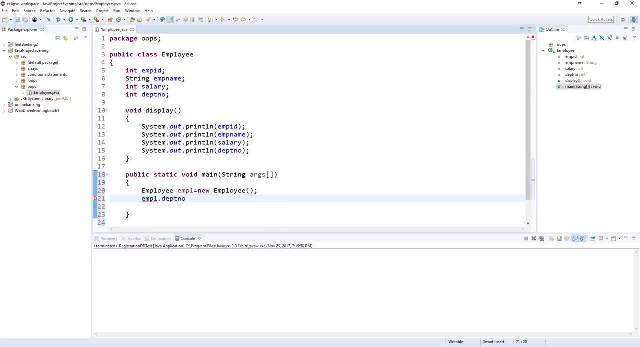 So just select this one DPT number. Let us take EMP ID first. EMP ID is equal to, let us say: 101 is ID. Similarly, EMP1 dot. EMP name is equal to some name and EMP1 dot- EMP1 dot, salary, some. 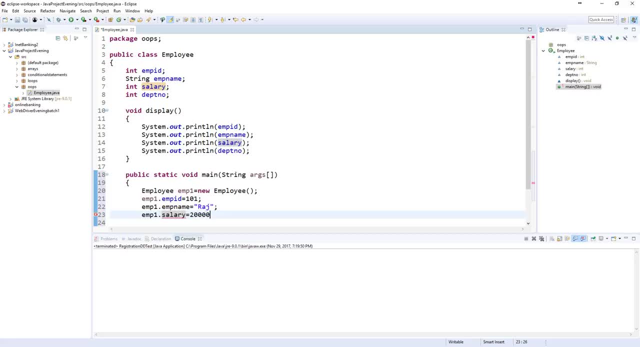 value, some number and EMP1 dot department number is equal to, let us say, 10.. Now these values are belongs to EMP1, employee 1.. Now, values are already assigned. Now, if you want to display these values, I can call this particular method. 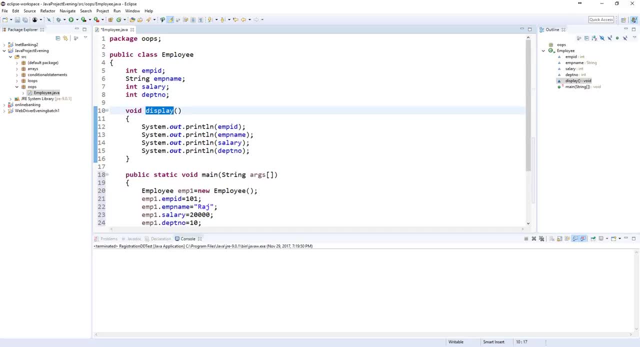 Display method is also belongs to the same class, right? So if I create an object, through this object, we have access to this variable. similarly, we can also access this particular method: display method Now, EMP1 dot display. it will automatically pop up the methods and variables. 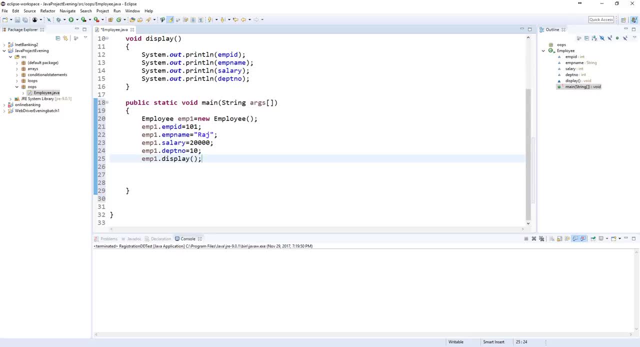 Okay, Now execute this. It will give you all four values Now. similarly, I can also create different number of objects. Now I will create one more object, one more employee right. EMP2 equal to new employee. This is an object for another employee. is the first employee. is the second employee. 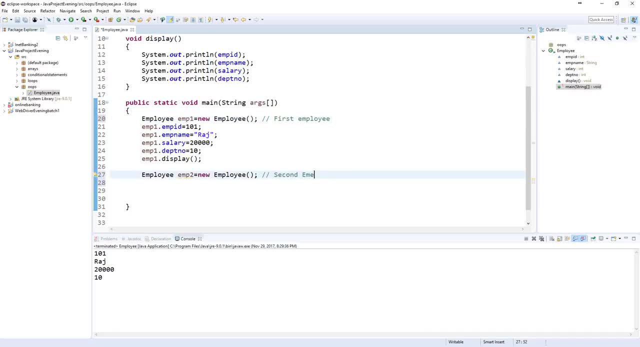 Okay, So now EMP2 dot. EMP2 is having its own ID name and everything right. So EMP2 dot again. EMP ID is, let us say, 102,. EMP2 dot, EMP name, some name and EMP2 dot. 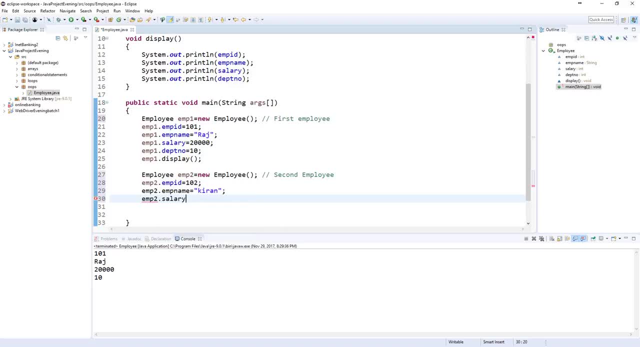 EMP salary: Salary equal to salary. EMP2 dot department number is equal to 20.. So this is EMP2.. Now, when I call this EMP2 dot display method, this method is: belongs to EMP2, right? So it will display only EMP2 values. 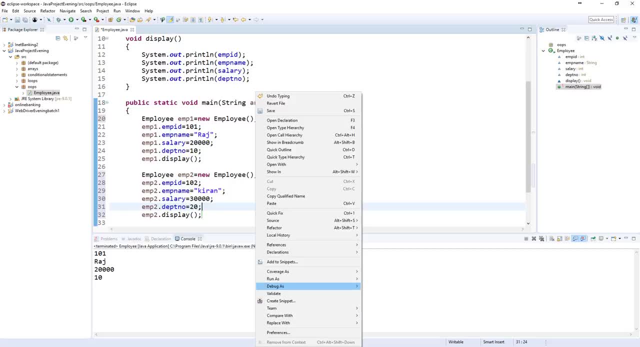 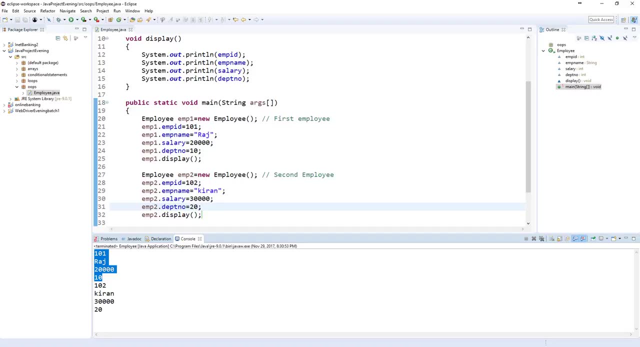 Now execute this. So first four are comes from EMP1, these are the details belongs to EMP1, and these are the values which are belongs to EMP1.. Okay, So this one is different. So all these details are sharing by every object, but still values are different from. 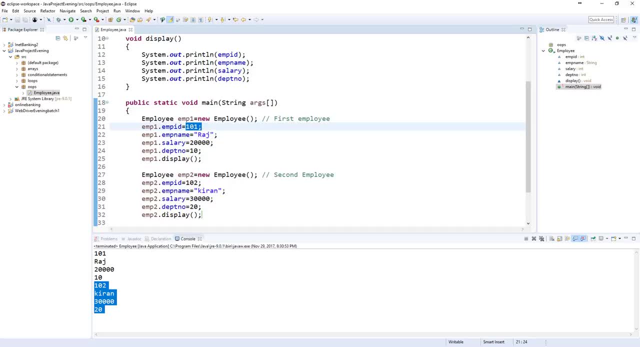 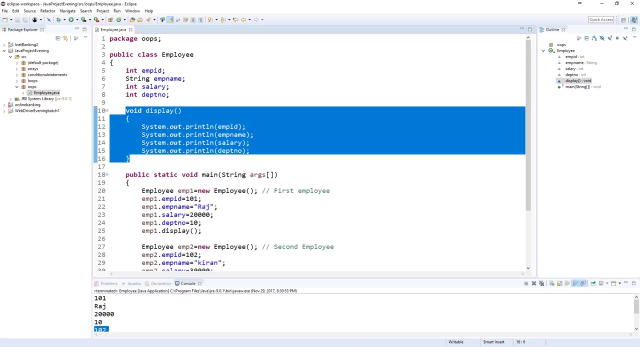 one object to another object. This is a very important point we need to understand. Okay, So for what we have done is we have just created a simple class which contains some variables and some method, and then we have created an objects for the same class and, through 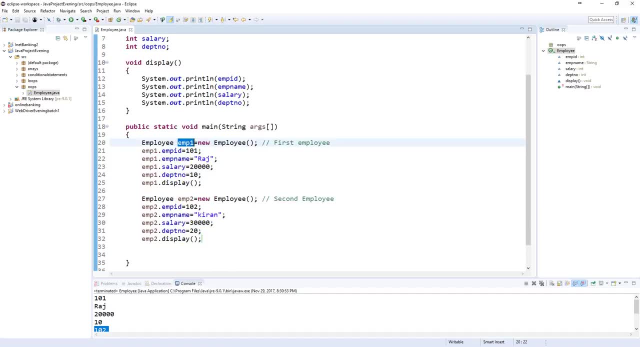 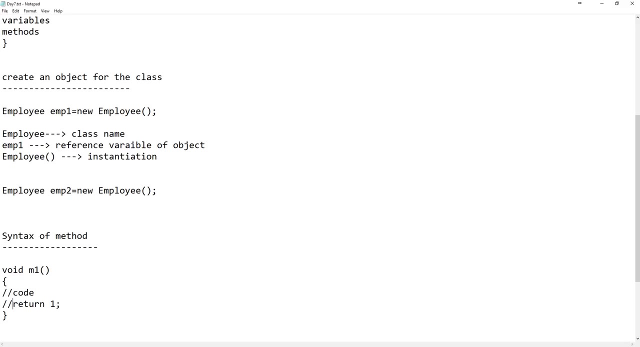 objects, We have access to those variables or we have assigned some values to those variables, And also we have called that method, which is also belongs to class through object. Okay, So these are the important points. Now, these points, we have covered. 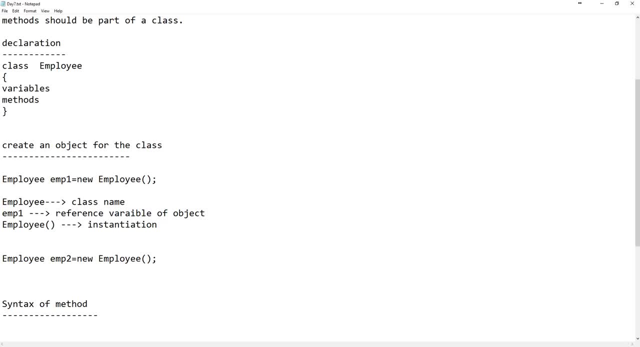 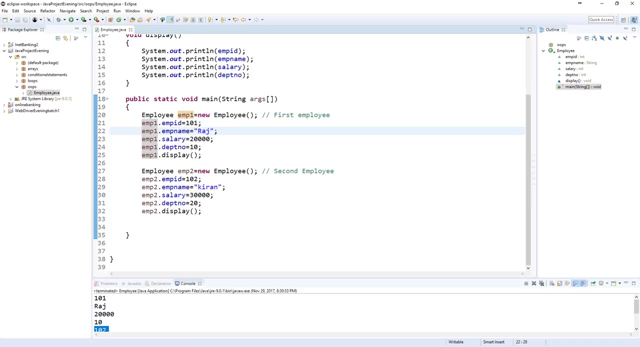 So how to define the class, how to define the variables inside the class, how to define a method, how to create an object and how to call those variables and methods by using object. Okay, Okay, Now I'll tell you. now we understand what is class and what is an object. why object? 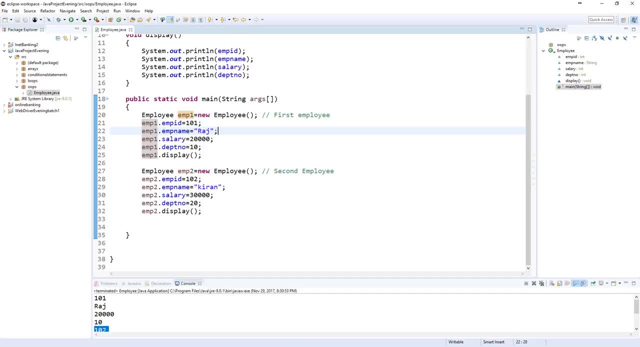 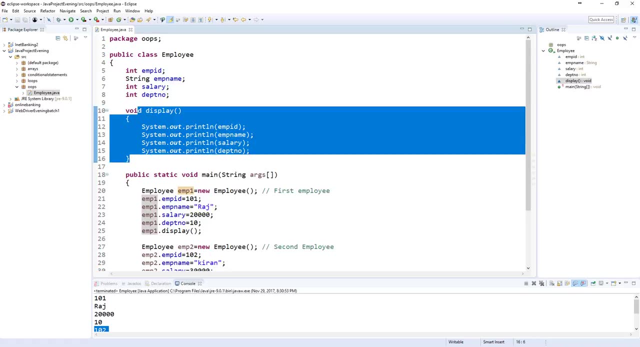 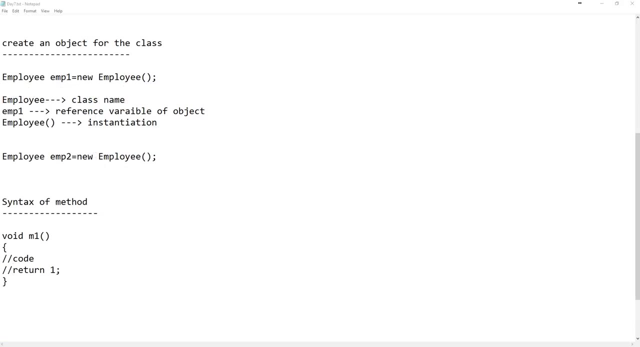 is required. why object is required? because if you want to access these variables and methods, we have to create an object. Okay, Now let us talk about the methods: Methods. So here we have also methods. What is method? So in this class I already defined a method called display method. 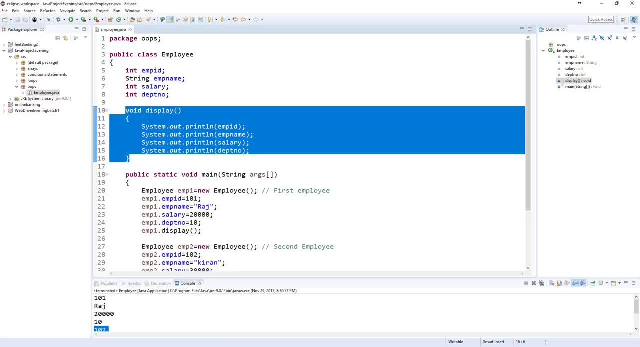 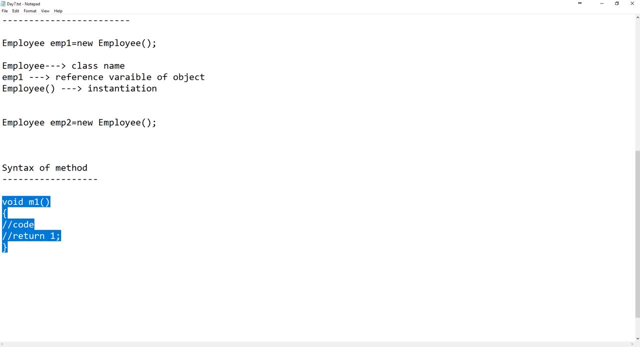 And I already told you a few points. A method may return some value. sometimes method may not return value. So if you see this example, this method is not returning anything, So that I put as a void. So if you observe here, even display is not returning anything, just it is printing those. 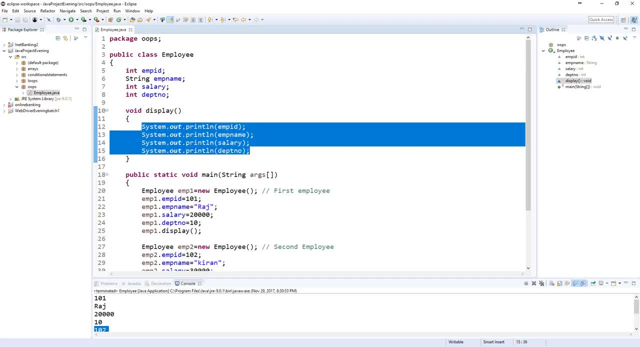 values. So in front of this method I specified as a void, Now I'll tell you different types of methods. So here, before going to explain types of methods, let us understand in how many ways we can initialize these variables. So we have initialized these variables through object. 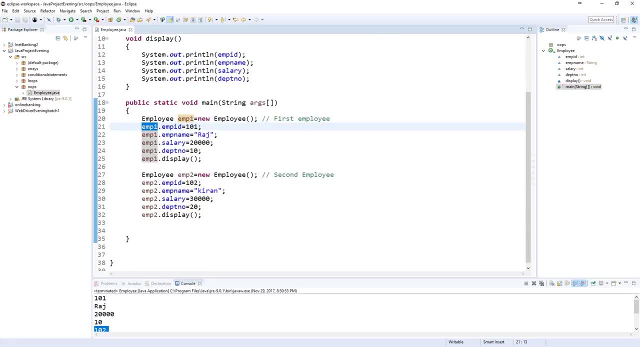 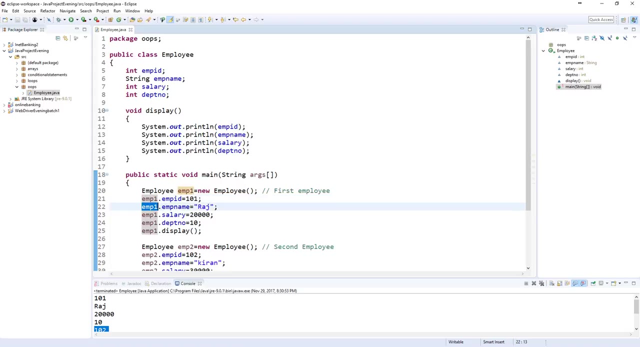 Directly. we have accessed these variables through object. Now we will see how many ways we can initialize these values. So there are three different ways we can initialize these values. Every object is having the same variables right, But the values are different. 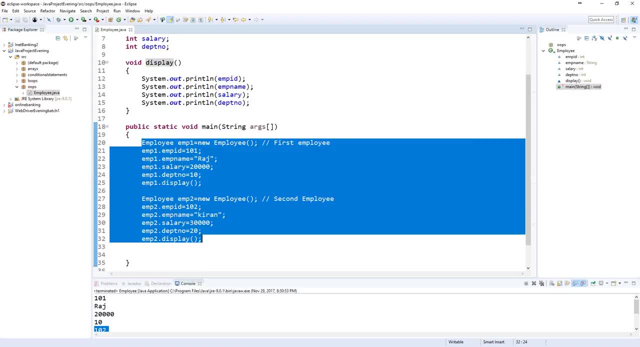 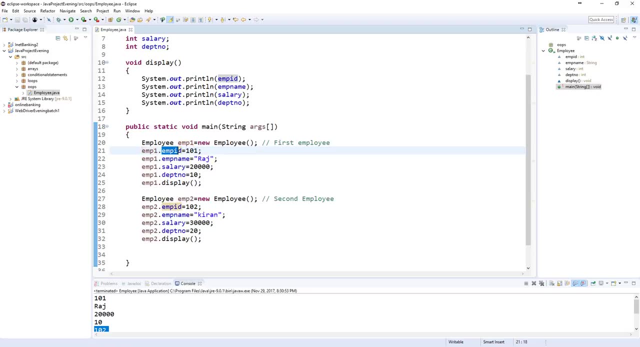 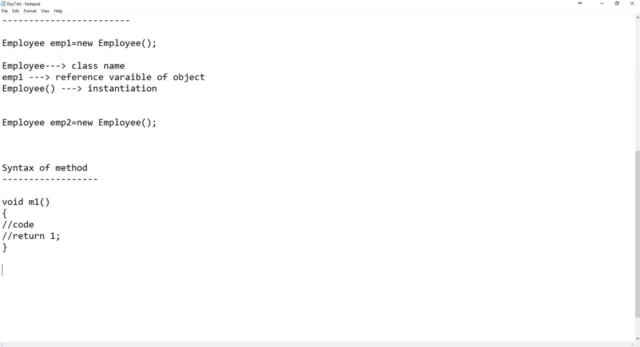 But in this particular method, we have assigned these values through object And through object we have accessed these variable names and then, directly, we have assigned these values. Now let us see a few more methods. How many ways, how many ways we can initialize the values to class variables. 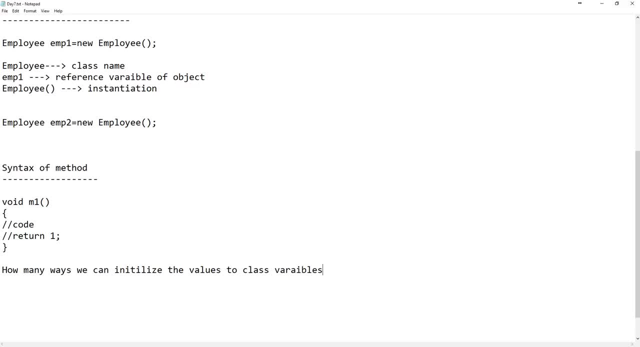 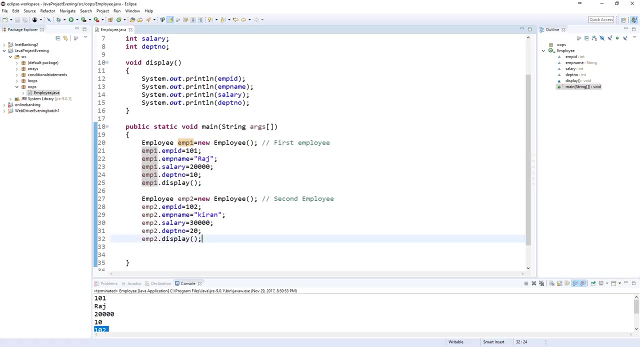 Okay, How many ways we can initialize the values to class variables. The first way is using object. using object, this is direct method, directly that we have seen. now. using object, you can access this variable name. we can assign this apps. we can create any number of objects like this, but every object is independent. 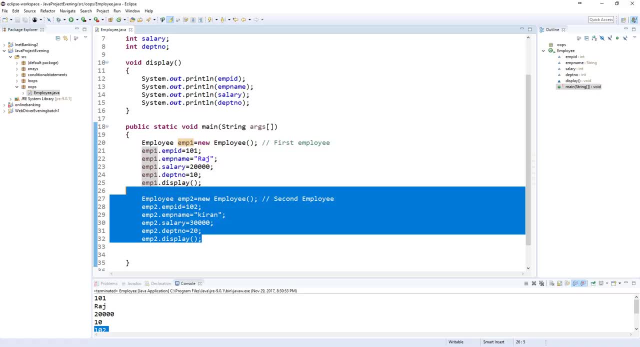 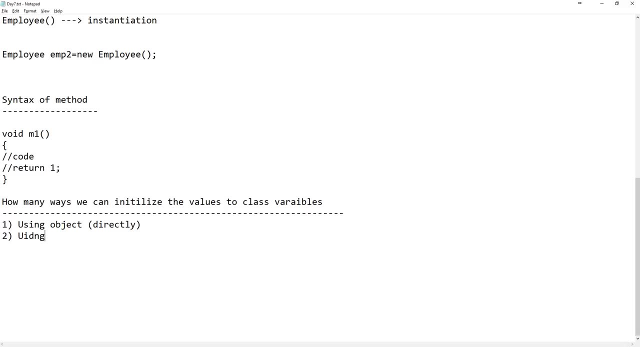 this is the first method. now there are few more methods. second method is using constructor. I'll tell you what is constructor. third method is using method. so using object, using constructor, using method. so these are the two, three different ways we can initialize the class variables. so now, first method, we 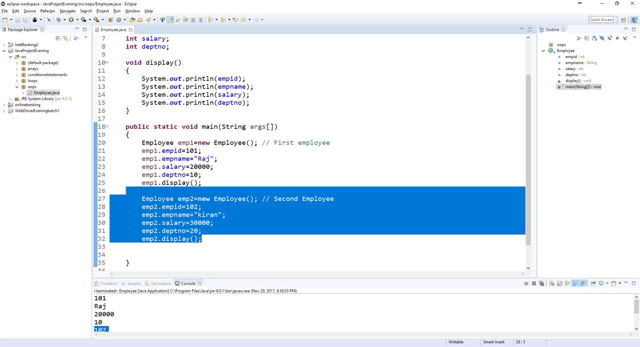 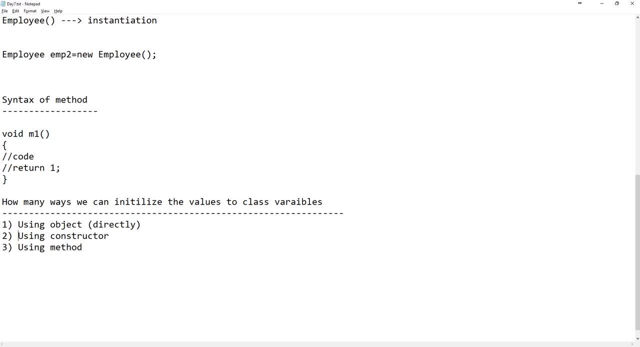 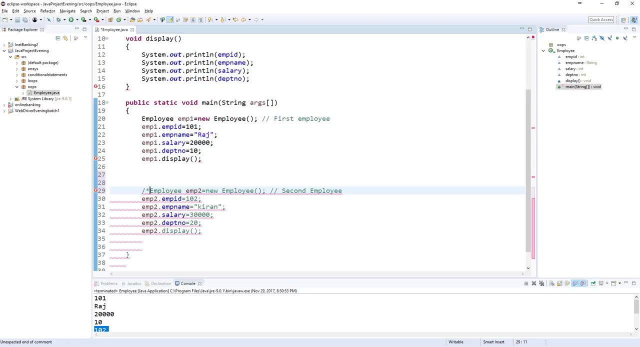 already see. so directly we can access this object, specify the variable names and assign these values. now I'll tell you the second method, using constructor. so now, let me just sometime, I'll comment this code. okay, I'll comment this code now. this code will not execute at the runtime. now what I will do is what is. 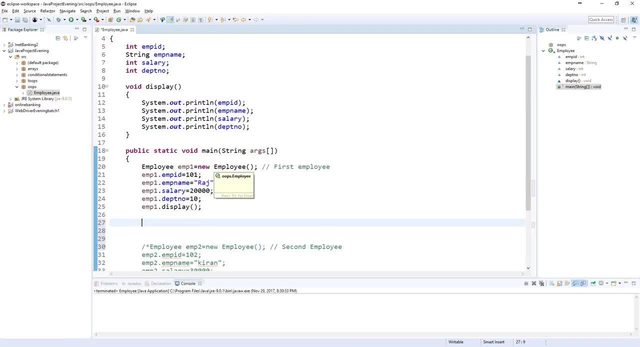 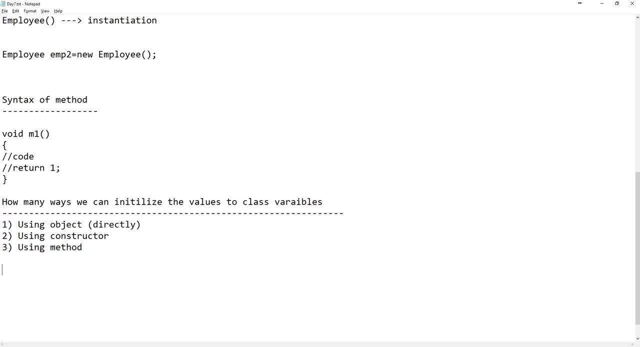 constructor. constructor is also a method. here I'll give you a brief introduction about constructor, but in detail we will discuss in the coming classes. okay, because constructor is a big concept. so constructor is a kind of method, just similar to a method. the difference is: but the constructor name should have same name as class. so whatever class name we have, 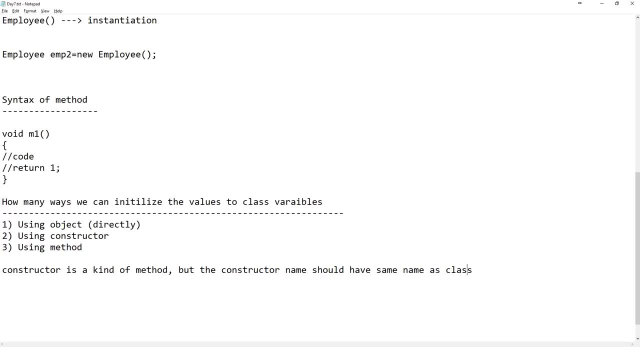 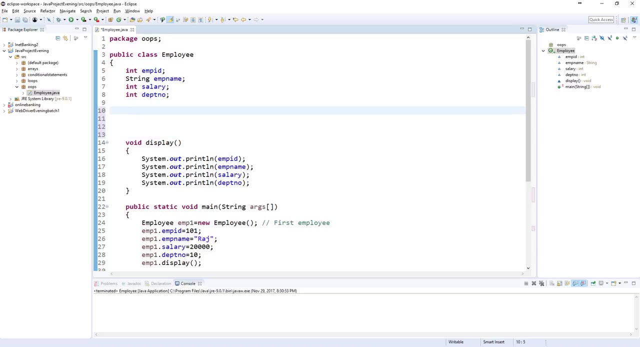 specified the same name. the construct is also should have. that is one fun, and the constructor is a kind of a method just in like a normal. okay, now, inside this class itself, i will create one more method here, so i will name that method as the same class. i will. 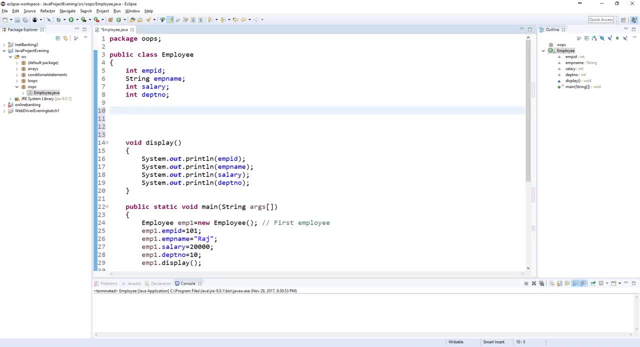 give the same name to that particular method as employee. now i will create one more method with the same name, called employee. this is my constructor. this is my constructor. so if i define a method within the same class with the same name of the class, that is basically called as. 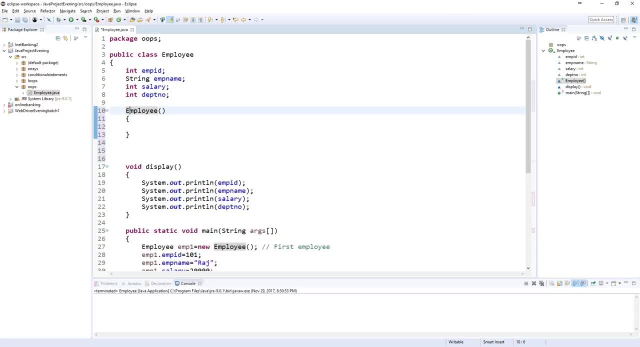 constructor. so now, this method, what i will do is: this constructor will take some parameters. let us say some parameters. what are the parameters? let us say first parameters: integer type, that is id. the second parameter is name, that is string type, string name. and the third parameter is: 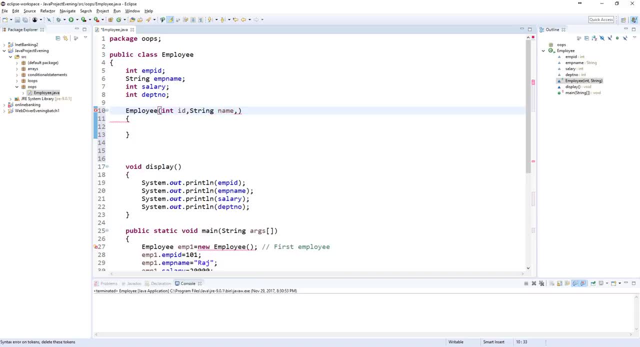 again into type, into cell. fourth parameter is again integer d number. so now this constructor can take some parameters and these parameters we will pass later. okay, so this is a constructor. basically, employee is a constructor because the name of this method is same as a class name. so whenever you see methods with this name as same as class name, 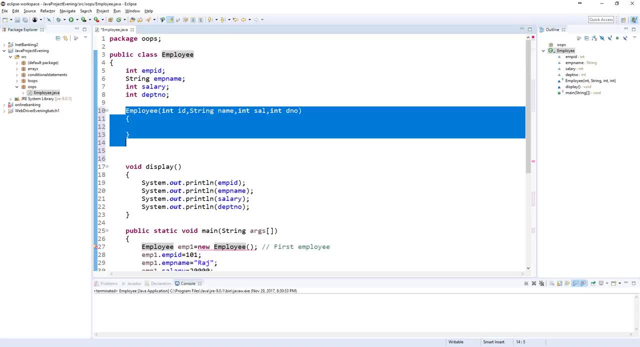 that is a constructor that is basically called as constructor. now this constructor is taking values or some parameter from outside. we will pass these parameters at the end later now. these values: id name and salary department number. these values we need to assign to these variables inside the constructor. now emp id equal to id. right, so now emp name equal to name. 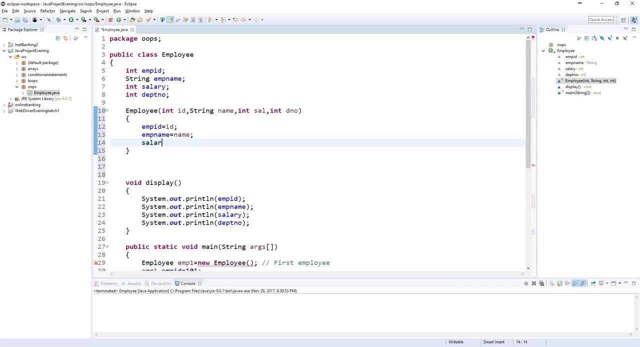 salary is equal to cell d. pitch number equal to d number. now, just, i have just initialized the values, i haven't done anything else. i took these variables from outside. the values will come later and those values, whatever values are there in id name, salary, department, number. the same values have been assigned to the class variables emp: id name, salary and department. okay, 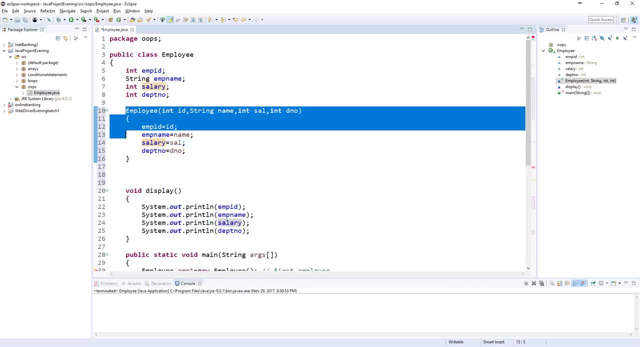 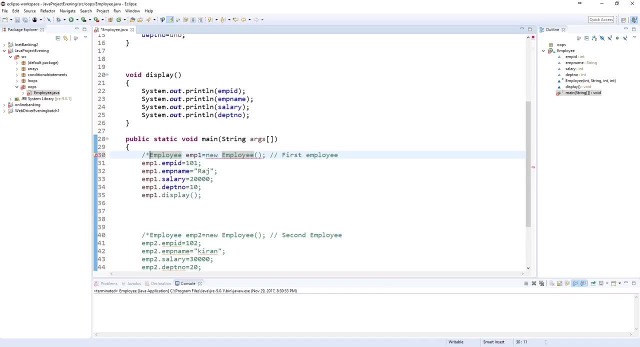 this is a constructor. now, instead of assigning these values like this- i will also comment this part, because this is the first method. okay, this is the first method. i'll come and write one more comment- is a assigning values to class variables using object. this is the method one. 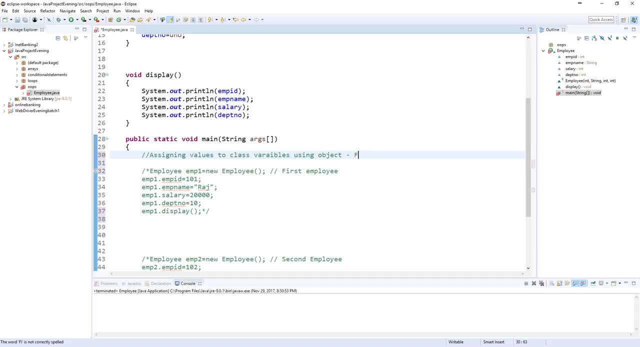 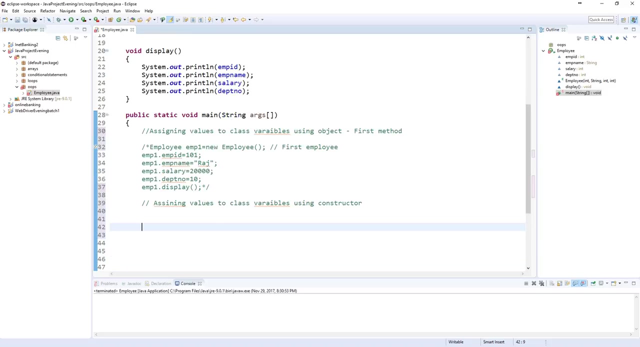 this is the first method i have shown. okay, first method. now, this time i'll show you assigning, assigning values to class, variables, variables using constructor, using constructor. so how to use the constructor. so we already define a constructor within a class. now only thing is we need to call this constructor. how to call this. 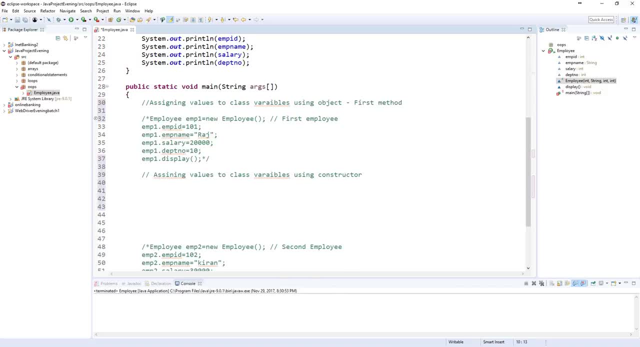 constructor. constructor will automatically called at the time of object creation. here also, we need to create an object, but we don't use object for initializing values. okay, so how to create an object: employee emp1 equal to new employee. this is how we need to create an object now, at the time of initial. 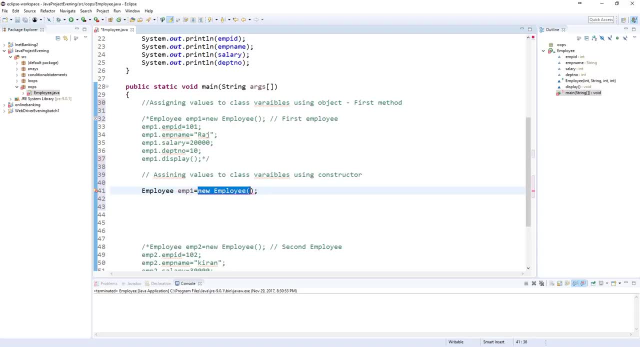 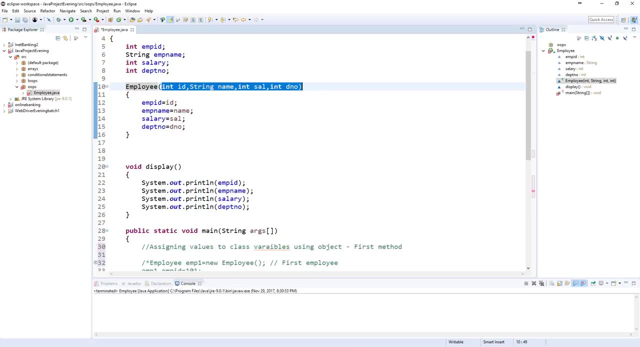 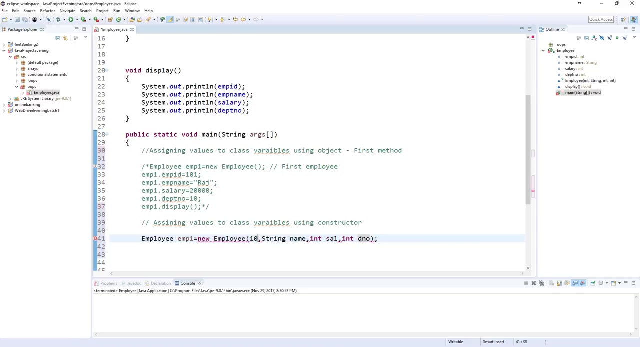 instantiation. we need to pass those values. so the in the same order. so employee is taking the same order, parameters right in the same order. we need to pass the values. so first one is id. we need to pass let us say one zero, one is id, next one is a name. should be in the double quotes. 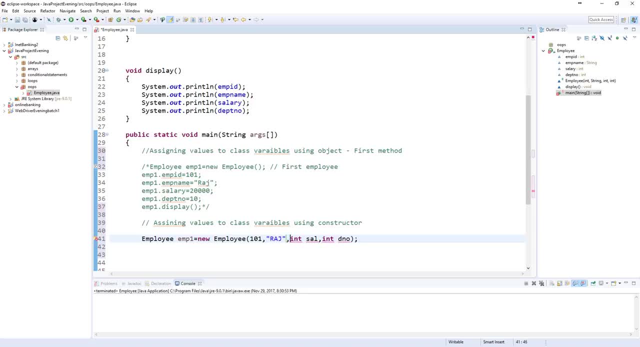 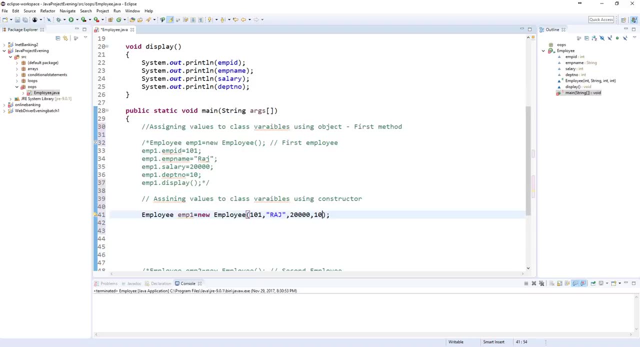 next one is a salary value. so salary value, you should also use salary value. you should use salary value, then department number, that is 10. that's it. as soon as I created this object, I need to pass these values to the constructor. so what is constructor now? constructor is a kind of method. 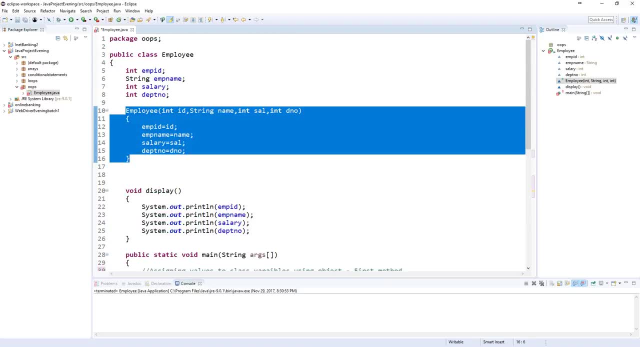 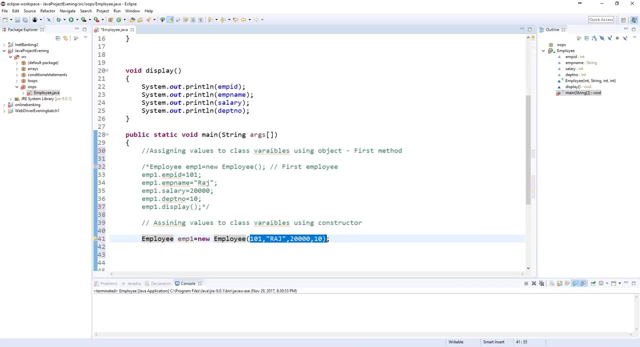 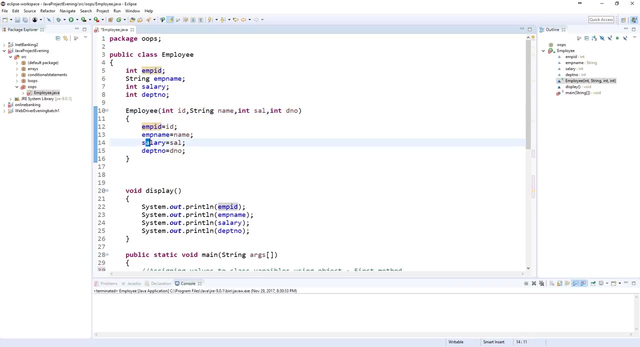 which will have the same name as class name, and this constructor will automatically called or invoked at the time of object creation. okay, now these parameters will be directly assigned to here: ID name, salary, department number- and these values are again assigned to EMP: ID name, salary and department number. now, values are ready. now we need to display those values. for that we 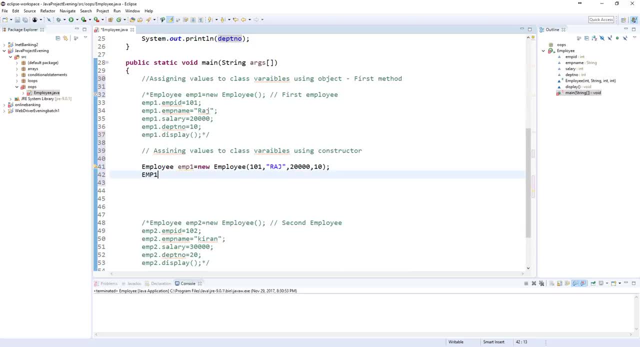 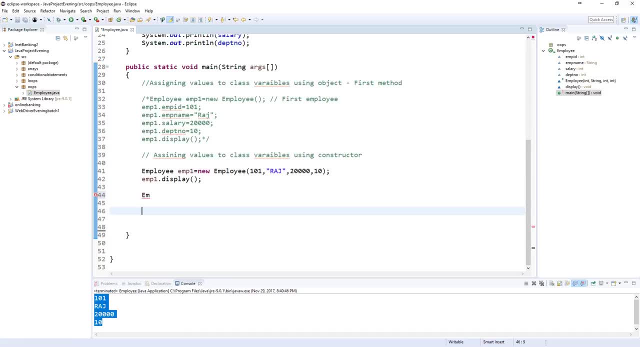 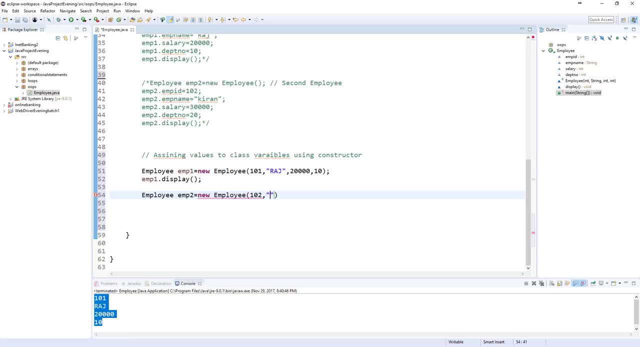 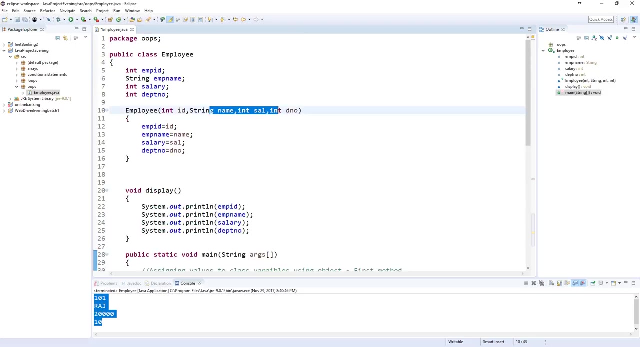 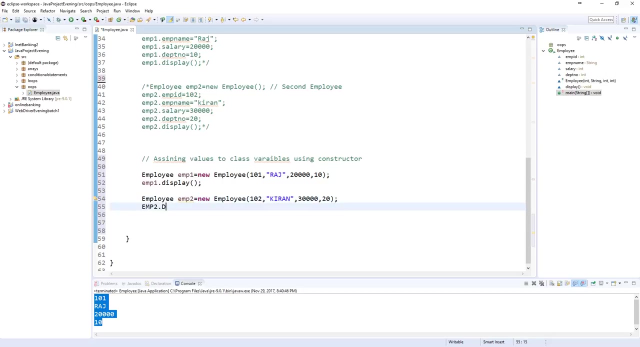 let us say name some salary and department number. that's it. so this is another object. Now these values are again assigned to these variables, and assign those variables and then assign to the class values. Now, through this object, EMP2 dot, I call display method. EMP2 dot- display method. now this will give you: 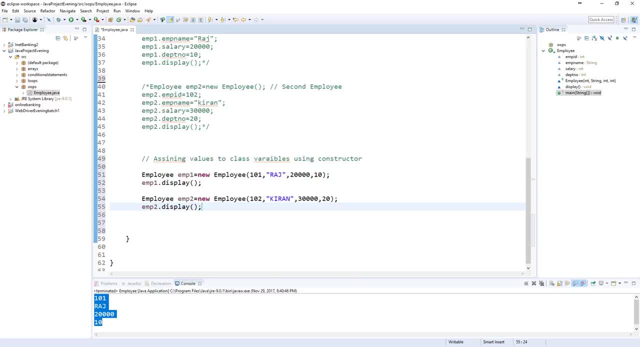 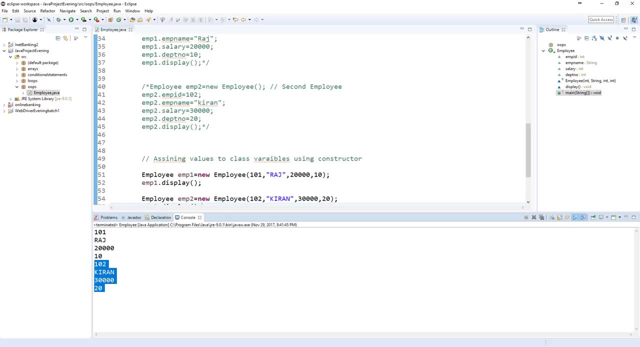 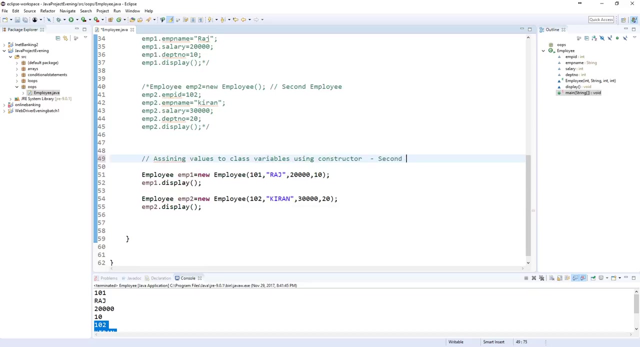 details of employee 2. Run this, it will give you the details of employee 2. So this is a method. 2, So assigning the values to a class variables using constructor. this is Second method. This is second, So using constructor. so now how we need to constructor. 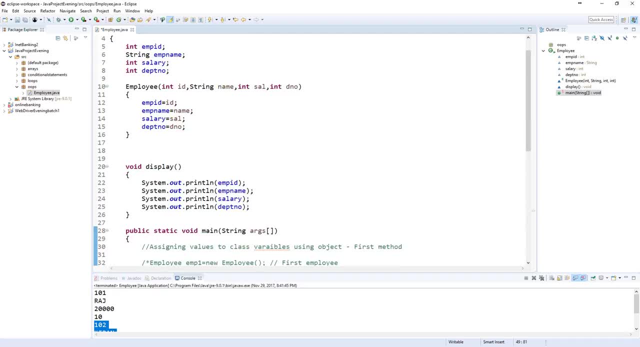 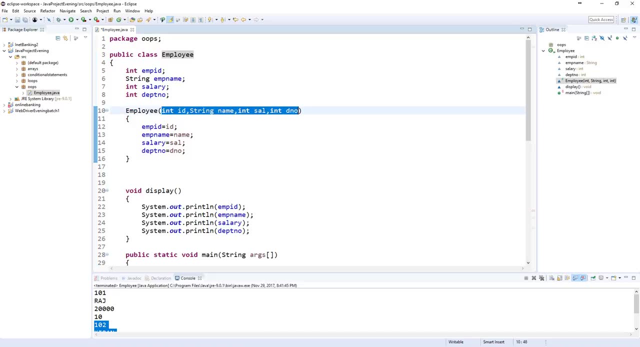 We have to define one more method with the same name of the class team and this method will take some parameters. But in the well, when we define the parameters list, We have to specify the Data type and the variable name. data type and variable name. data type and way. 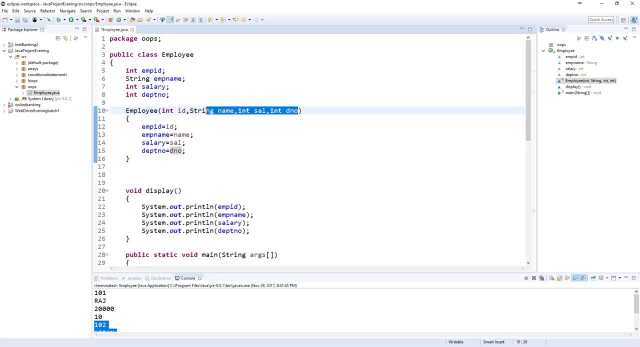 So this is how we need to define So here. if you observe, I have used different names here. Why? because These names are already defined in the class. right? if I say EMP ID here, can we define like this: let us say: if I say EMP ID and. 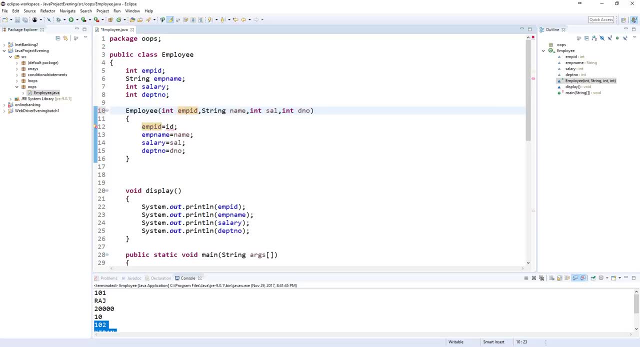 There is some issue here like this, because it cannot identify this. suppose if I say EMP ID again here like this, This will show something wrong at the runtime Because this constructor doesn't know which EMP ID comes from outside, which EMP ID is comes from, comes from the class. it will confuse. 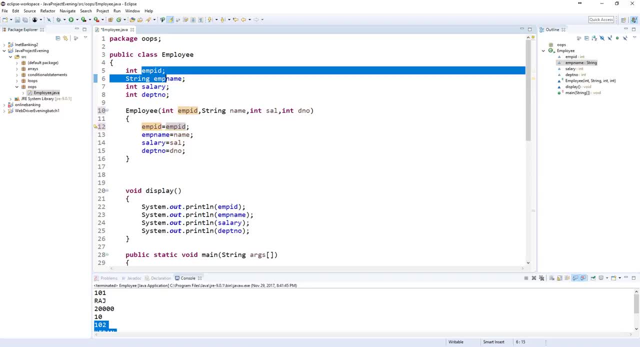 So that's the reason I have mentioned as a different name here, Let us say ID, so some different variable name should be. But this is a actual, normal format. but still, if you want to use the same variable names, still you can use. but there is. 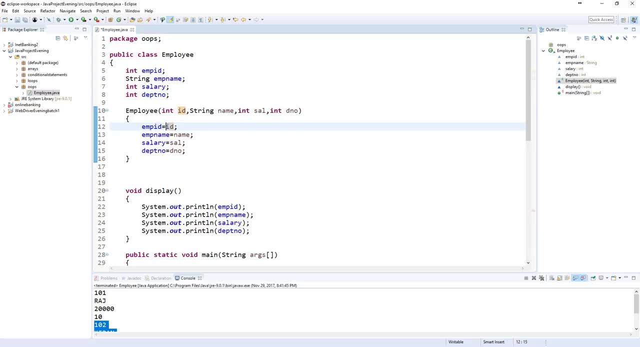 This keyword is useful. Okay, so I will talk about this keyword later, But as of now, just remember this: if you want to, if you want to get those values from outside, We have to define the data type variable, data type variable, data type variable like this, by separating commas and the same variable values. 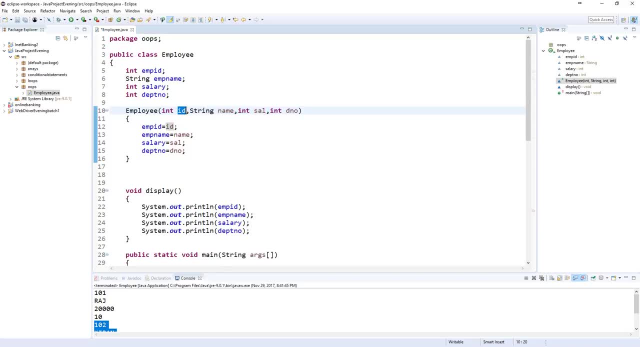 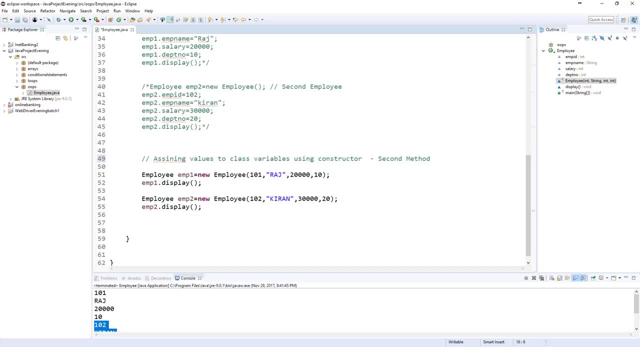 We need to assign to the class variables. This is a constructor. now how to call this constructor? at the time of object creation, We need to pass some parameters. Then it will automatically. Constructor will be invoked. the values will be initialized to those where variables. then we call the display method. 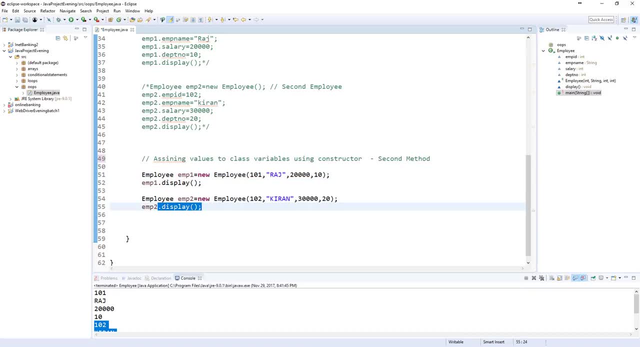 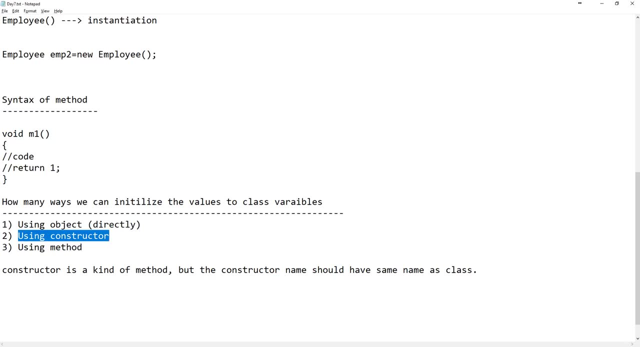 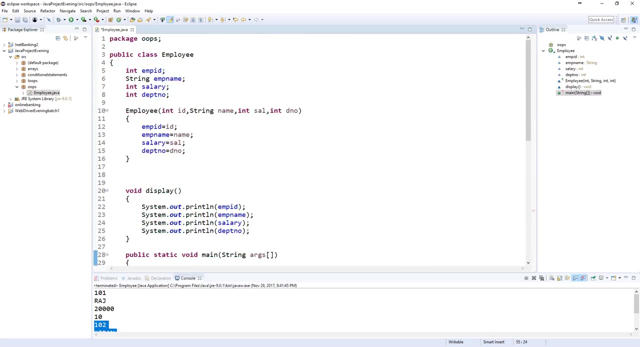 This is a second method To assign the values to those class variables. next one: Using method also. we can do that Using method also. we can do that now. for that, what I will do is the same class Display method is already there, right? I will create one more. 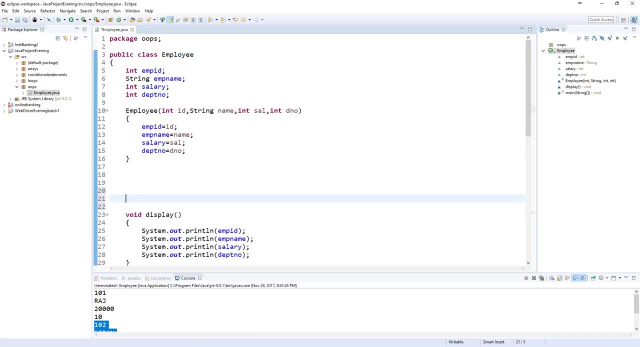 This is not constructor, This is a normal method. So method is, I'll say, set data. This is my method. Okay, set data. This will also take the parameters. I'll also mention this method. method can take the parameter, may not take the parameter. that is up to you, based upon your logic. 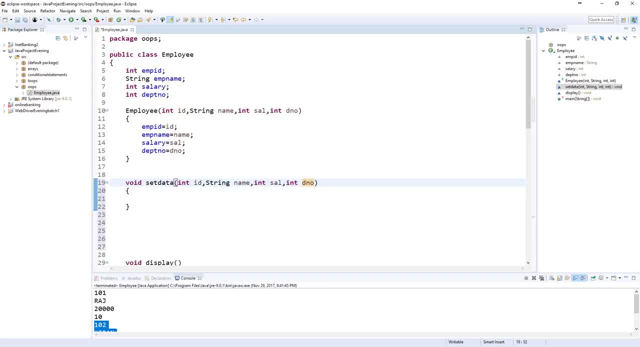 You can write your method. Okay, I'll discuss about the methods in detail in the coming classes. Okay, so here I'll define one more method. This method is taking some data. This method is taking some data: ID, name, salary, department number. now the same values will be assigned to the local variables. Now, again, I'll copy the same thing here. 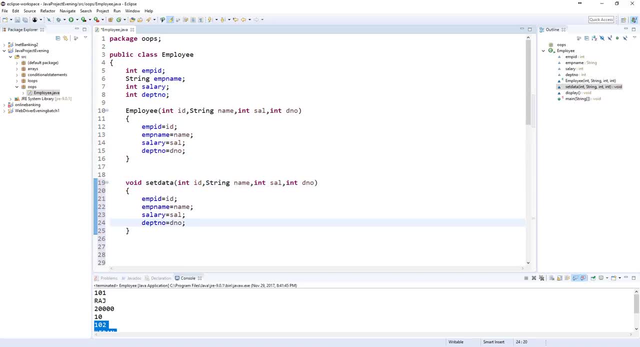 Okay, Now what this method will do. this method will take the parameter from outside and assign those parameters to the class variables. now, when I use this method, just Comment this constant not required. Okay, but this method is responsible for initializing the values to those variables And display method is responsible for printing those values. 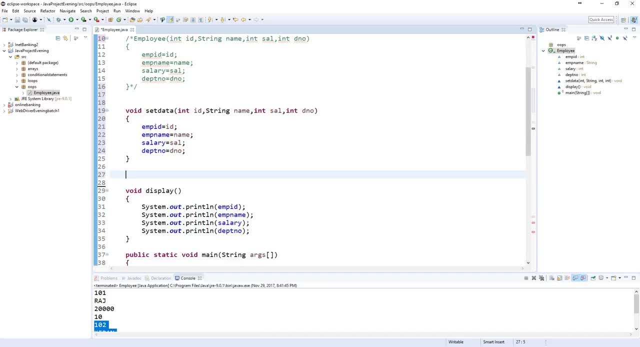 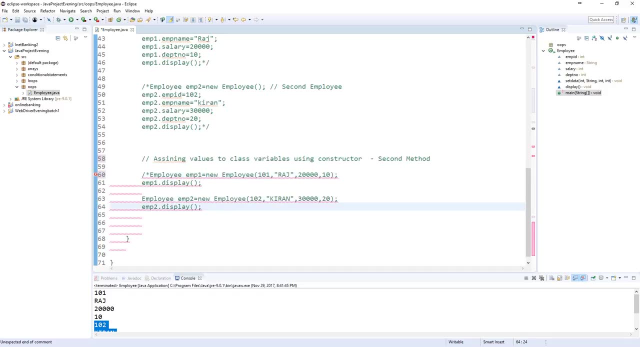 Now come back to your main code. now We have already seen the second method, right, Let me comment this now, the third method, Assigning values, class variables- using method Using method, is a third method Using method. now I already created one method, That is, set data. right now how we need to call these methods. 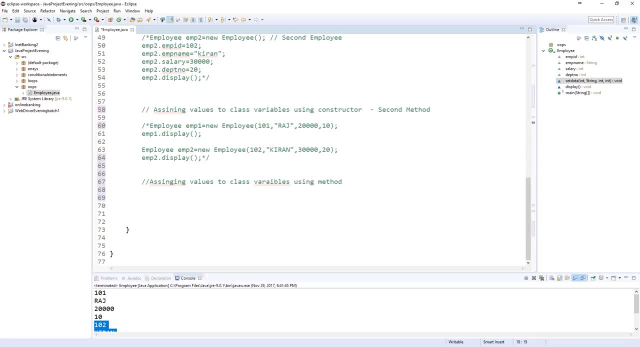 We have to create an object. without object We cannot call those methods. So, just like display method, we call right. Similarly, we have also called set method, set data method. but we need to pass some parameters. Now, employee is a class, EMP is an object. 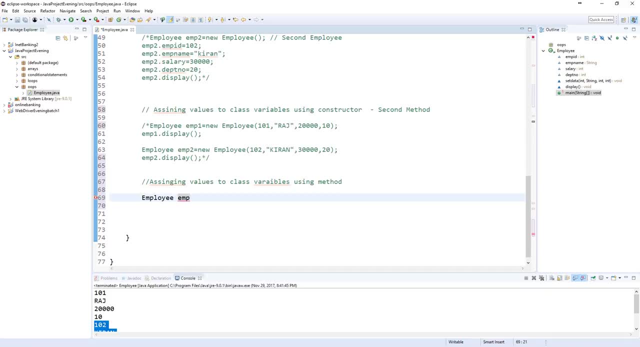 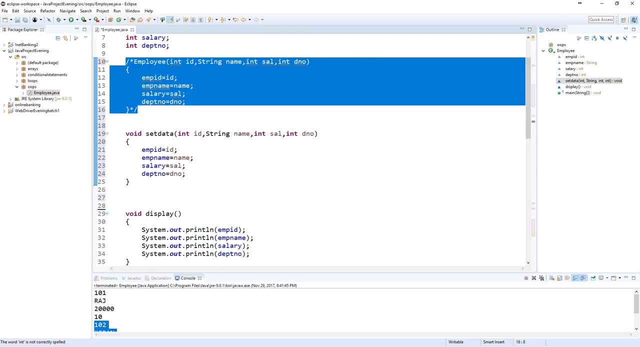 EMP one is an object equal to New employee. this is normal object creation right. But here we don't need to pass any parameter this time because we are not calling constructor Constructor. I already Commented, so I haven't executed this constructor this time, So I no need to pass any parameters now. 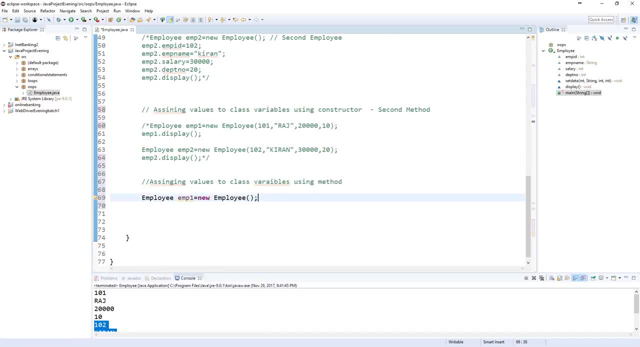 using this object- MP one dot- I will call Set data method. This is a new method. I have created a bow right, So this method I will call. if I want to call this method to object only it is possible. So EMP one dot- set data. 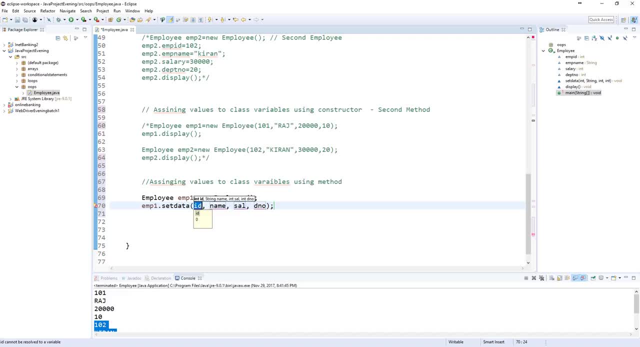 First thing, ID we need to pass. Second, name we need to pass, and then salary and then department. So this method we call. so as soon as we call EMP one dot set data, these values are assigned to. Here set data method will be called. these values are assigned to each individual variables. 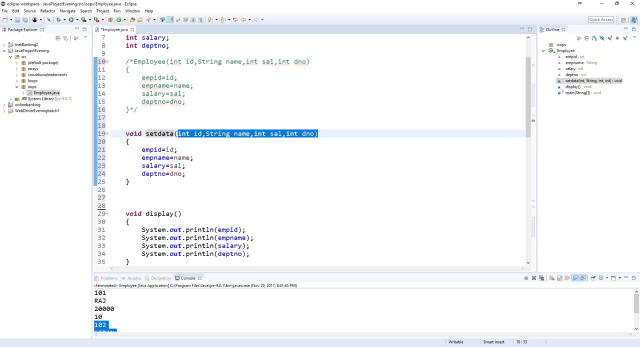 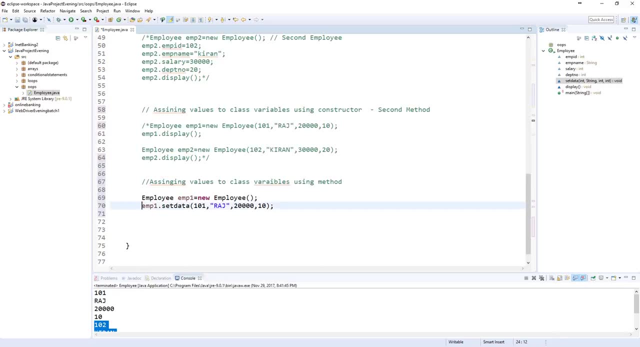 And then again these values are assigned to the class variables. So once we call this method, the values are ready in the variables. now we need to print those values. EMP, one dot set data method. We have, anyway, other method called display method. So this limit are not taking any parameters. if I call display method, that will just print the data. 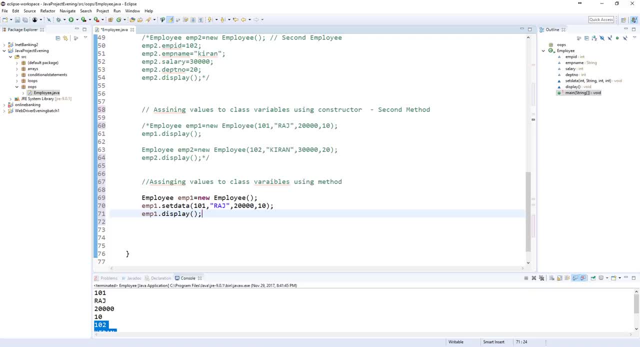 Which is what we stored in the variables. right, That's so. set data method will assign the values to those variables. Display method will display the values up from those variables. now execute this from mass navigation. Now you can see the same output you can see Now. similarly, I can also create number of objects. 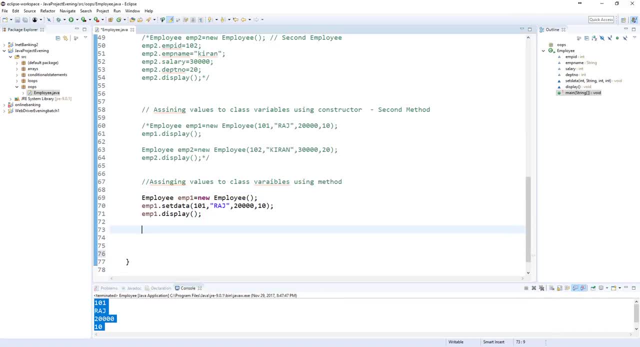 Let us say employee employee, EMP two: equal to new employee, Right. This is another object. now EMP two: dot. again I'll call set data method. This is a Different object. EMP two data is different right. So here I'll say one, not who. 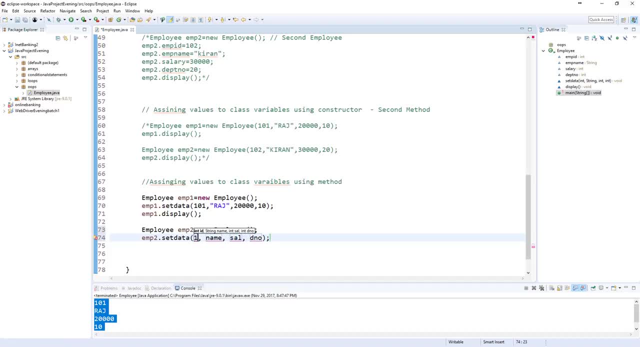 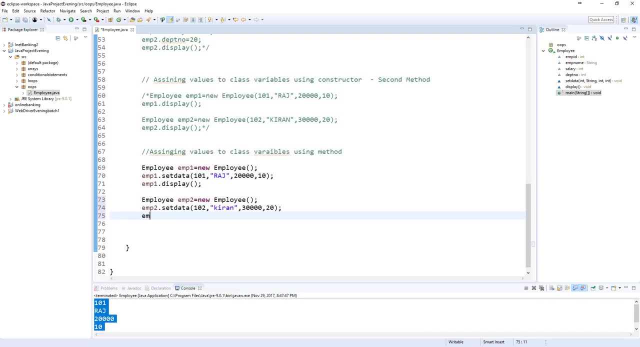 name is something different and Salary and Department number: this is different object. now, as soon as we assign the variables, we have to call method. What is that? display method: EMP two dot. Now, it's good this. Now we will get the values from both the objects. 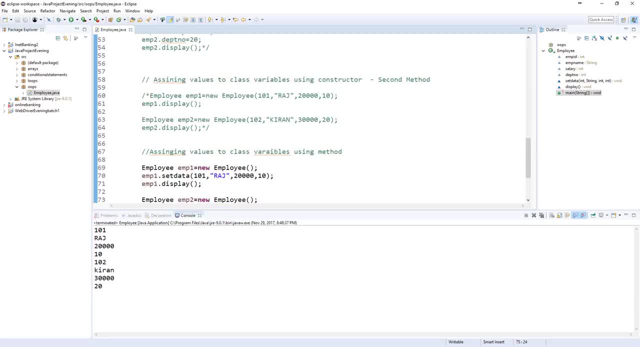 These are the values from employee one EMP one object and these are the details from EMP two object. So this is how we need to initialize the class variables: using method. Okay, so these are the three different ways: using object, using constructor, using method We can access, we can assign the values to those methods. 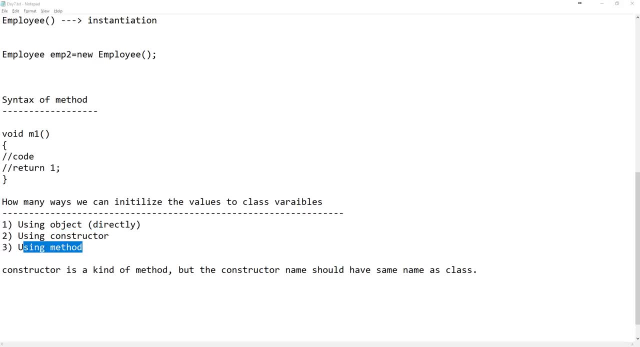 clear everyone. If you are clear, just confirm in the chart window, yes or no. So this is how. this is how we need to create the class object and assign the values by using Object, by using constructor, by using method. okay, Now. So now let us move on to. 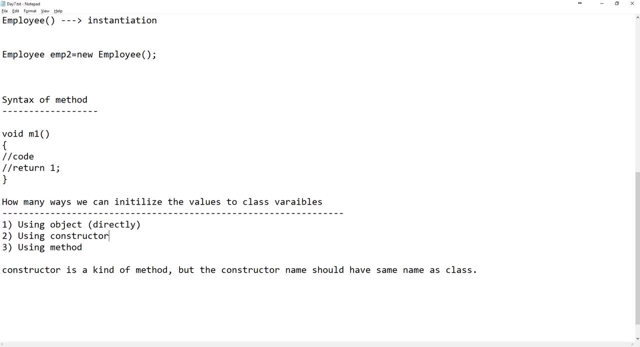 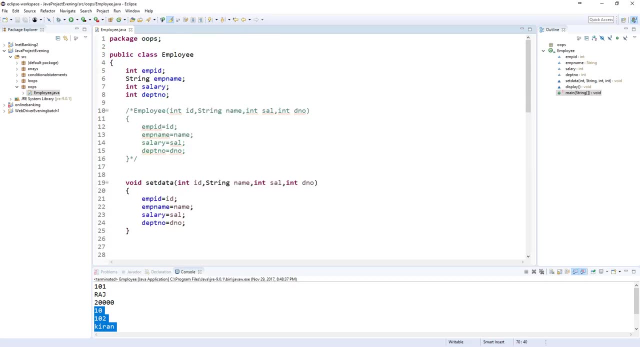 Methods in detail. So now, so far, what we have seen is how to assign these values to these variables in different ways, like through object. we can assign these variable values directly, or Through constructor- we can pass- or through method. we can do that, Okay, using method. This is a third method. 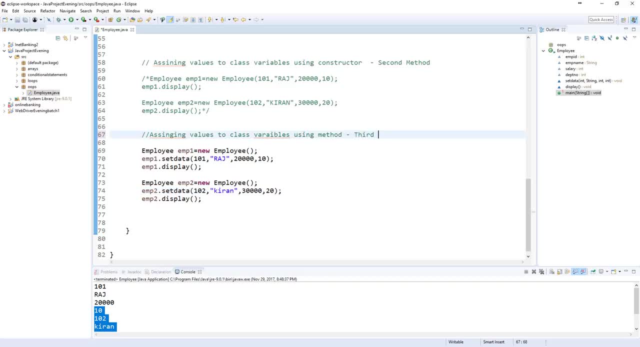 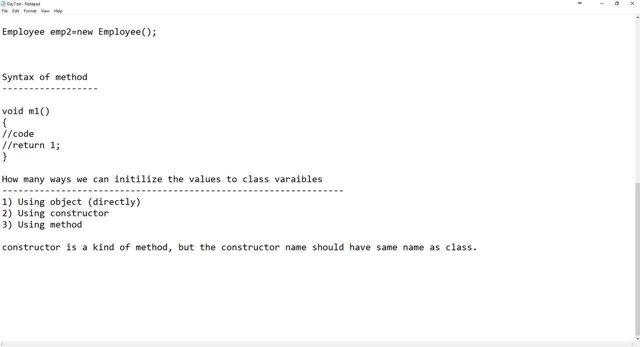 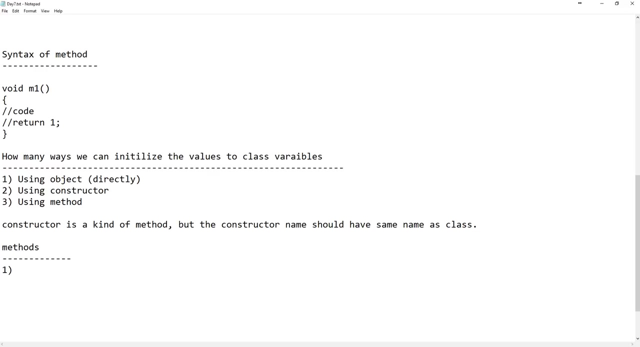 Okay, so now I will discuss about the methods. what are all different methods? we have methods So you can write different kinds of method. so sometimes there are four scenarios I will show you. Okay, If I define a method, Two things are very important. one is: Method may take parameters or method may not take parameters. That's the one thing. 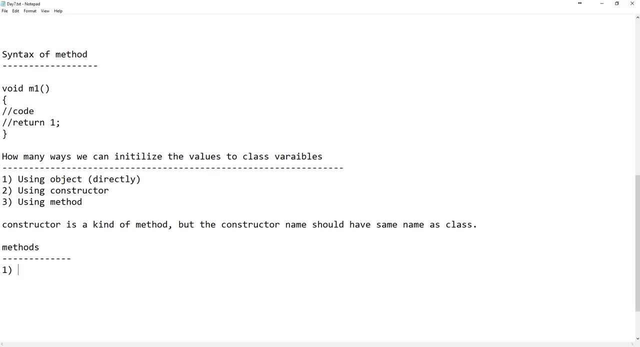 The other one is: a method can return some type, or method may not return some type. Okay, these are two things. So one is: if I define a method, If I declare a method, a method may not take parameter. sometimes it may take parameters, Example we already seen here. So set date, My method is there. So this method is some taking some parameters. 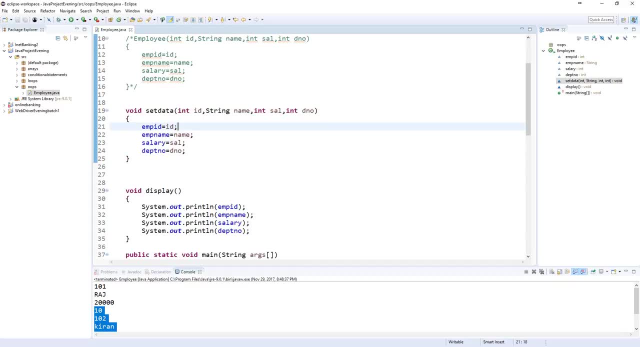 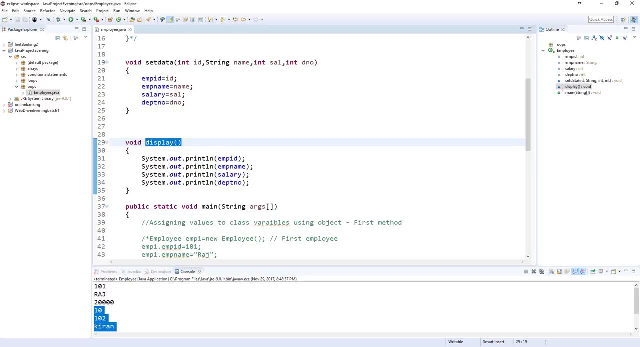 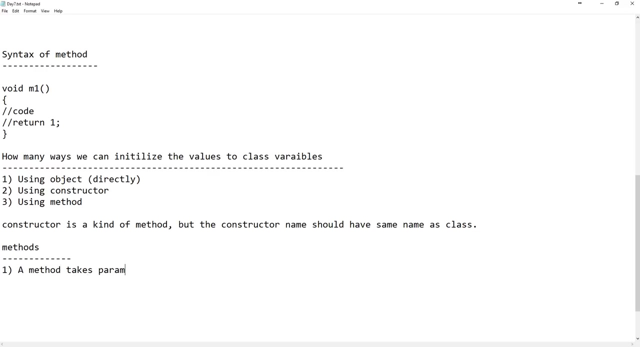 But display method is not taking any parameters. This is one example. So this is another case. a method Takes Parameters. there's a first, second thing: a method may not take Parameters. these are first context. these two examples we already seen and there is another concept: a method. 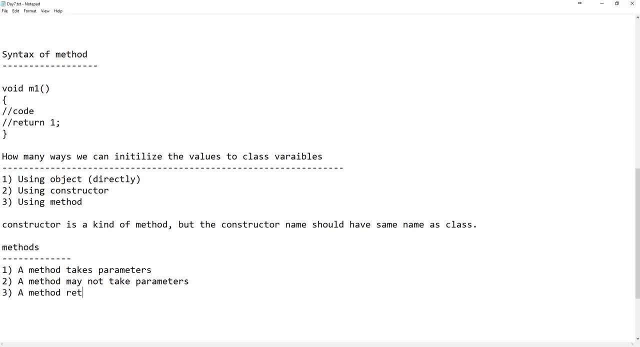 Returns. method Returns some type, some value or some value. It can be any data type and a method. A method may not return any value. So if you see this example- Set data method and display method- these two methods are not written anything. There's a reason we put inside this method as a void. void means it's not written anything. 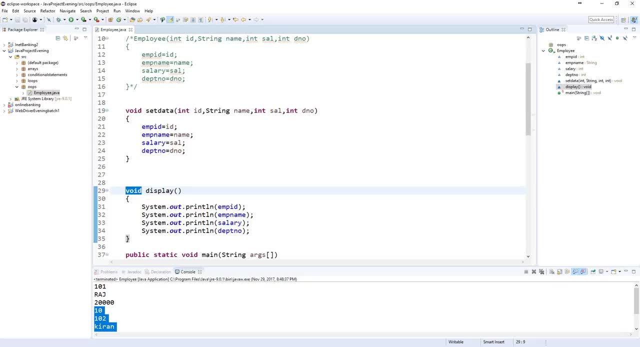 Okay, complete, empty. so Inside this method also, We haven't used any written statement. If I use written statement, you must specify some type here. Okay, so a method takes Parameters, a method may not take parameters. So for these two we have seen two examples. 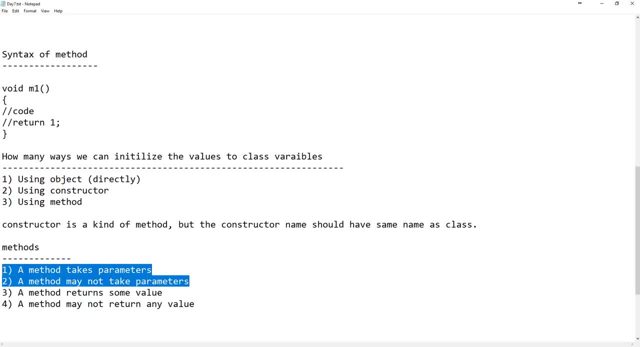 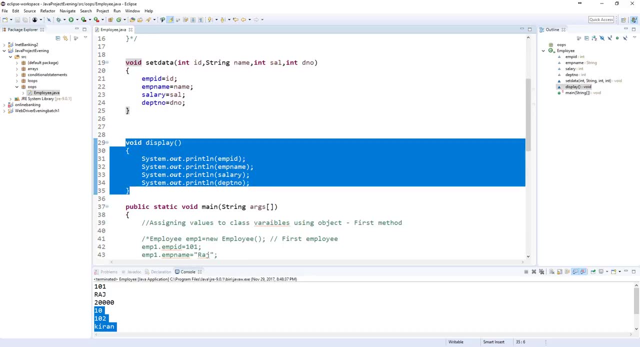 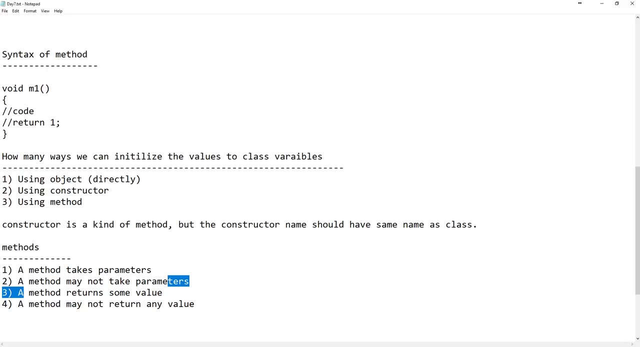 So, set data is a method which is taking some parameters. Display is another method which is not taking parameters. Now, a method written some value. a method may not return value, So, but both the methods we defined here are not returning any value, right, But there are some methods which will return some value. 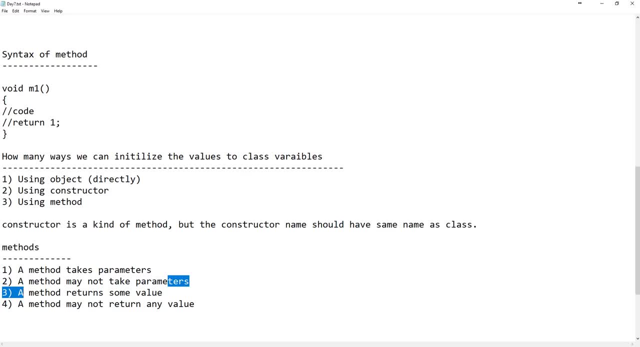 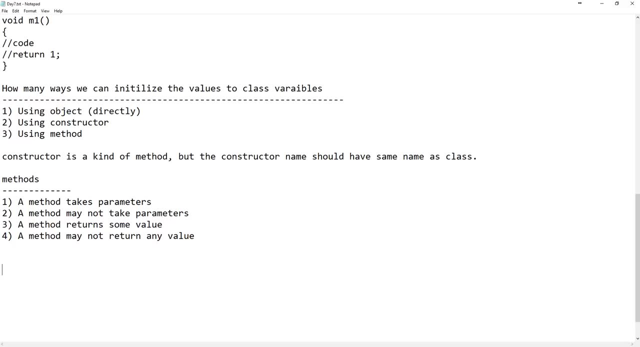 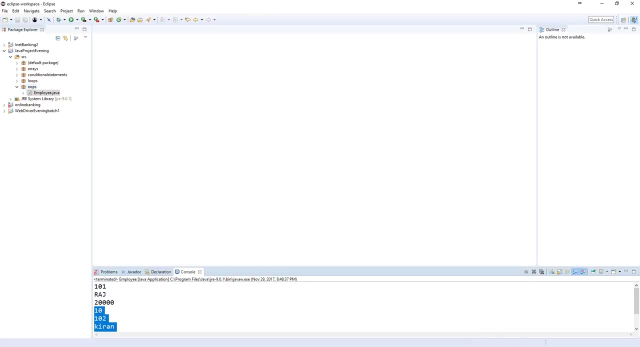 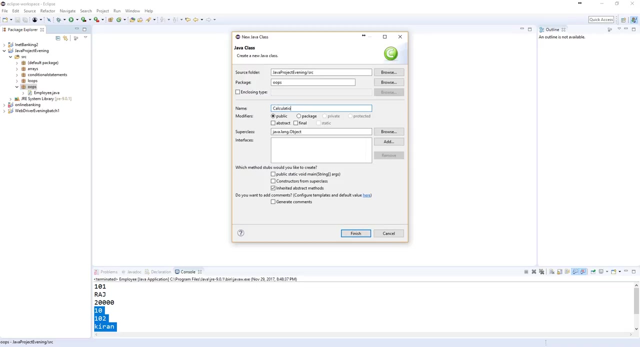 so in that case, how we can Define the methods For all these combinations? I will write one more class Example. I take one more example. So now let me create another class. Okay, so my class name is calculation. let us take main method. So calculation is my class and main is a main method within the class. keep this main method one side. 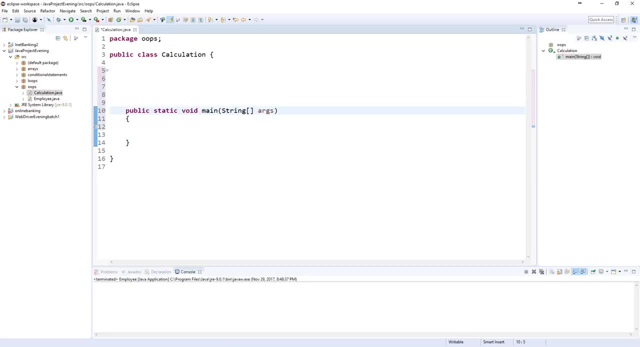 So, as I said, a class contains a variables and methods, right, So I will define two variables: integer a- Okay, and I'll define one more variable, integer B. There are two variables I will define, Right. So now here, I Will assign the values to these variables by using object. So how to create an object for calculation class. 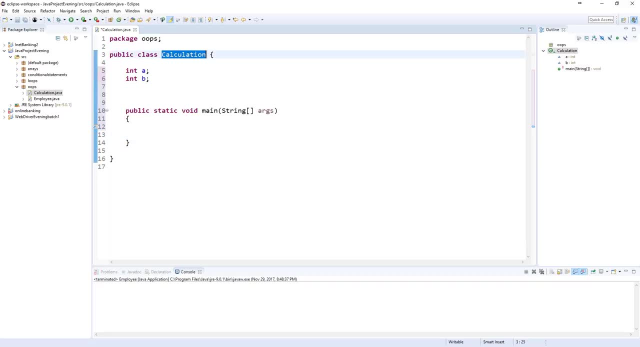 calculation. let us say Cal equal to new calculation. Now I have created an object for the calculation class, So using this object I can initialize the values to a and B. now I'll assign the values. Cal dot a is equal to 100. Cal dot B is equal to 200. 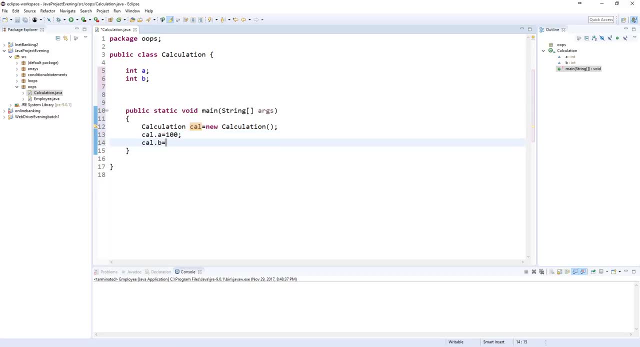 Now I have assigned two different values in a and B. Now I will perform certain calculation like sum of two numbers. So for that I will write one method here. Observe very carefully, I Told four methods. I tell, I told you four different things. a method take parameters. a method may not take parameters. 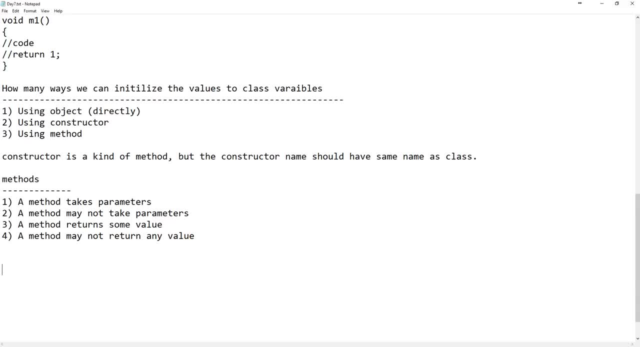 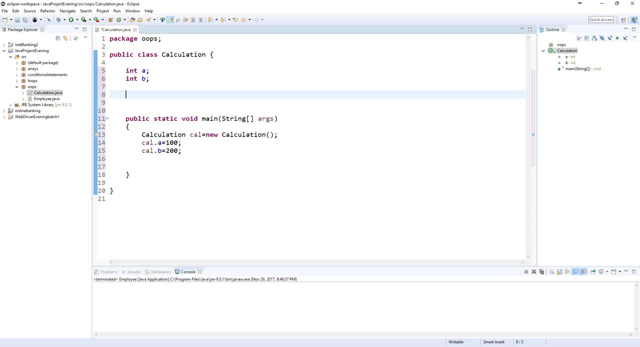 Similarly, method return some value. method may not return value. The first thing: a method takes parameters. So I will write a method: method Takes Parameters. so now, how do you write this method? I'll write method void Sum. method name is sum. This will take parameters. Okay, So for that reason, let us say int a comma. 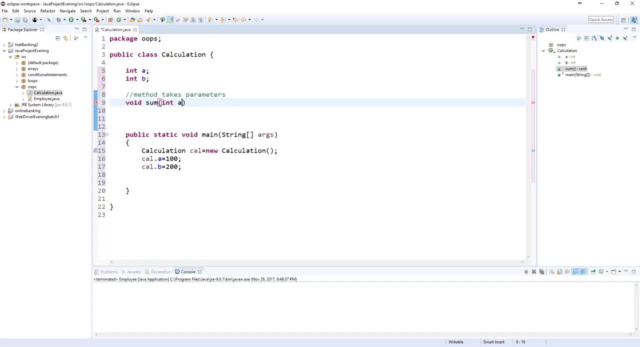 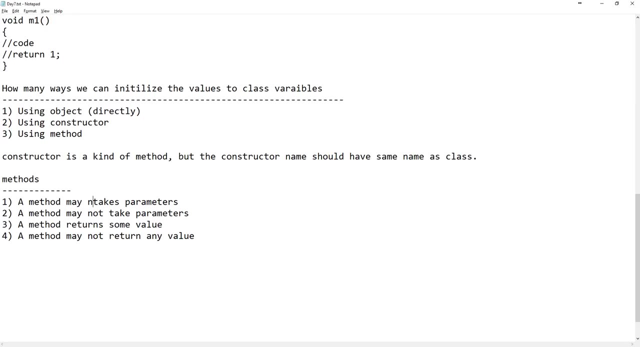 So first let us see without parameters. Okay, method May not Take parameters. The second one is: a method takes parameters. Okay, first we will see this one and then go for this one. So method may not take any parameters. So this method I will define without any parameters. now 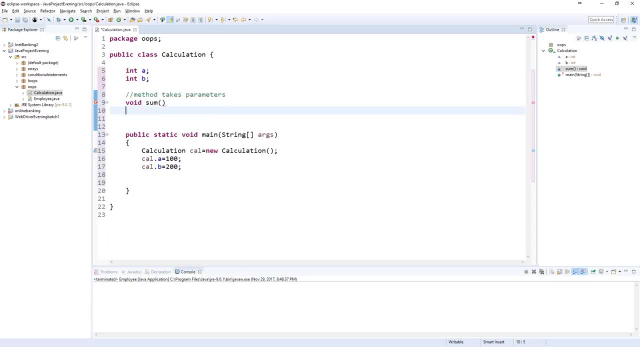 We already assign the values a and B. hundred to 200 is right. So now a and B is having those values. now here I'll print this value. So system, dot out dot. I'll say a plus. This is a code I have written inside the method. 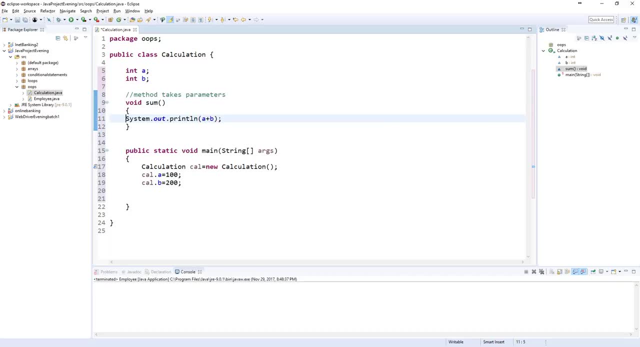 Now, if you observe, here I have a class which contains two variables and one method. What this method will do is it will perform the sum of these two numbers. now, if you want to access these variables and method, I Required an object, So I have created one object for. 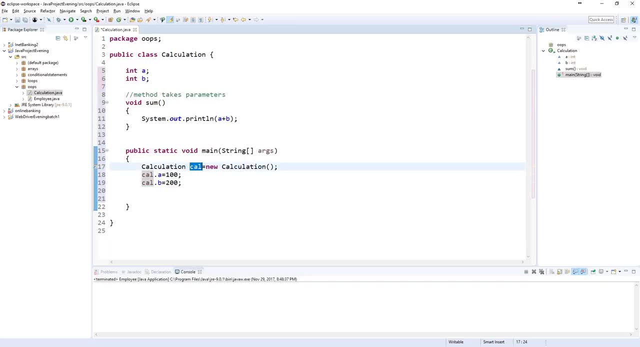 Calculations: class Cal: equal to new calculation. now using this object I have a sender: a and B values. now Cal dot sum. I call this method by using object. Now what happens? it will add those two numbers. now execute this. It will give you some of two number, that is 300. this is method. takes parameter the first one. 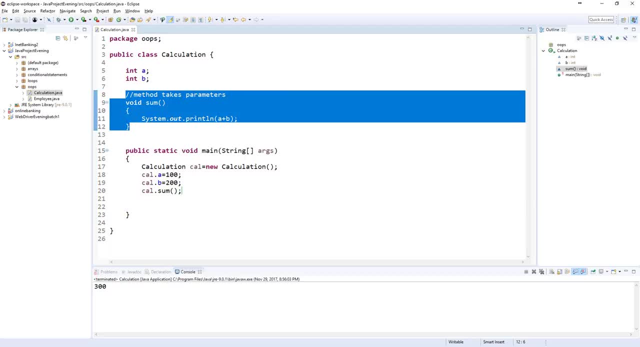 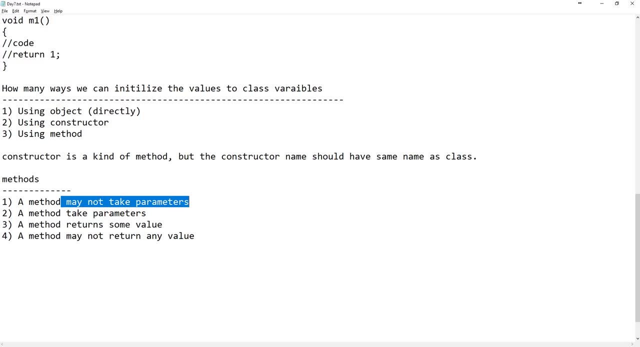 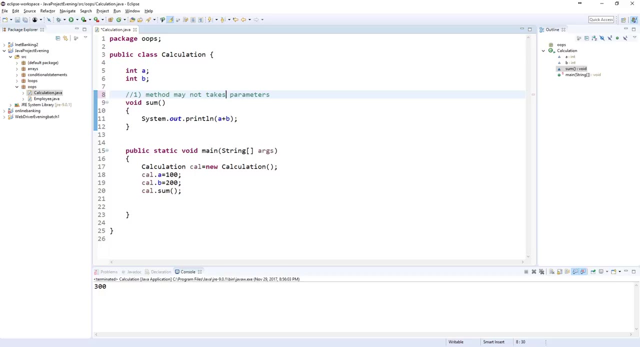 method- sorry method- May not taking any parameters, may not. It's parameters, empty parameters. We can say: empty parameters. Okay, this is an example for empty parameters. a method will take nothing, okay, It will perform just operation. this a first example. Now let us see second method: date parameters. 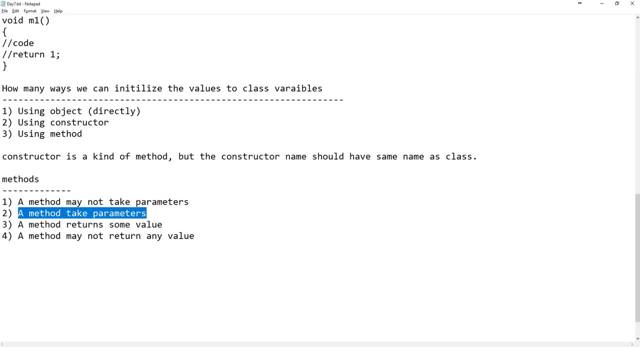 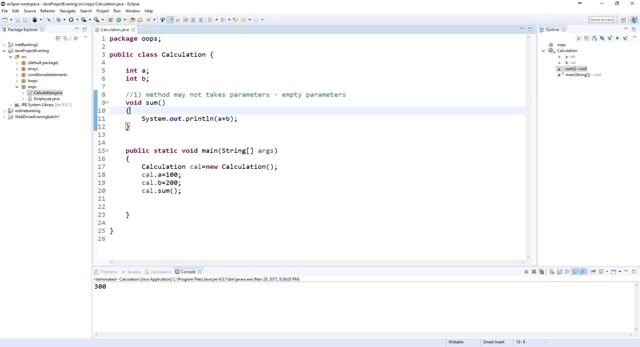 your method: date parameters. Now here, what I will do is I I will create one more method. I'll comment this first one. Okay, So a method. this is a second one. A method may take, or a method takes parameters. Method takes parameters. Now here I'll specify the value. 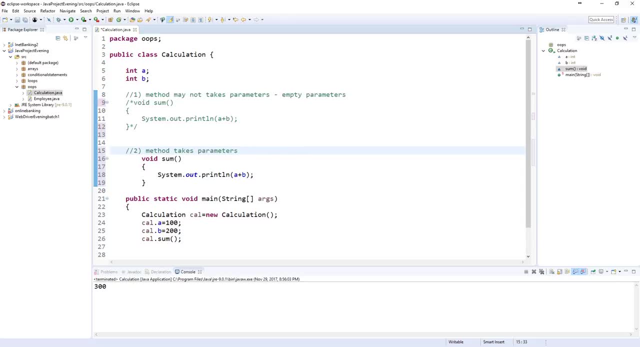 So int, let us say x, int. let us say y- Two parameters it will take And these x and y will assign to the a and b. a, b are the class variables, So a is equal to x and b is equal to y. Now here directly systemoutprintln: a plus b, I can directly add: Okay, This is another method I have defined. So this method will take parameters from outside. 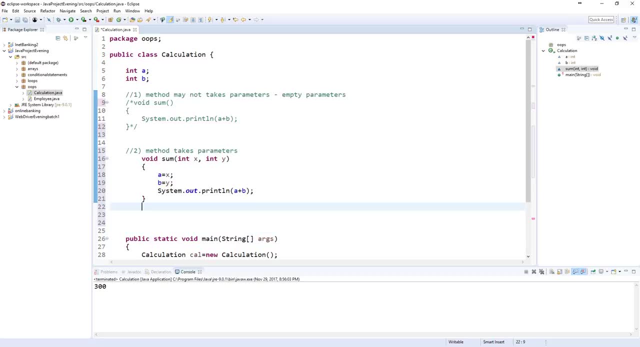 X and y will assign to the a and b And do perform the a plus b operation. Now, in this case we should not call like this: These are irrelevant. Let me comment this Because we have already created a method for taking parameters and giving the output. Both will do. Now, simply, what we can do is object. we have already created Right, Use that object. Okay, This is the first method. I'll say again: 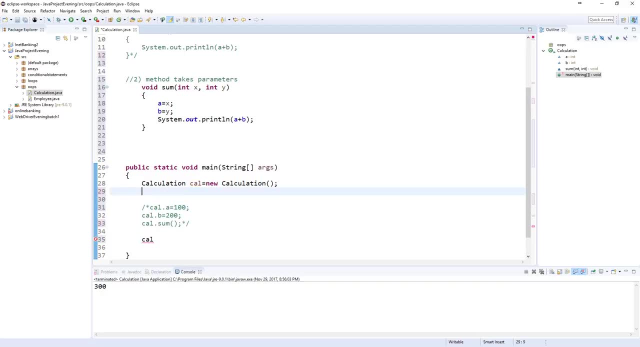 Don't confuse, Okay, So please. That's the reason I'm writing the comments here For the first one. If you want to call the first one, This is required. This method is required. Okay, Now I'm going to the second one. 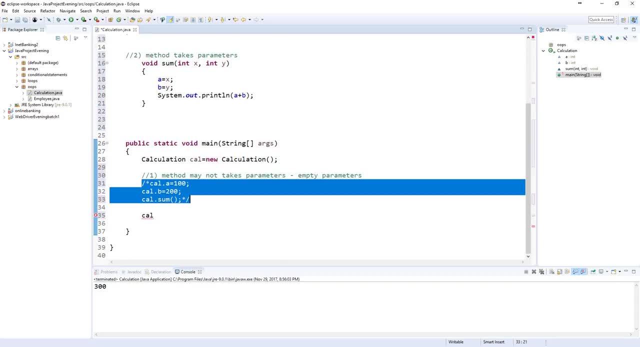 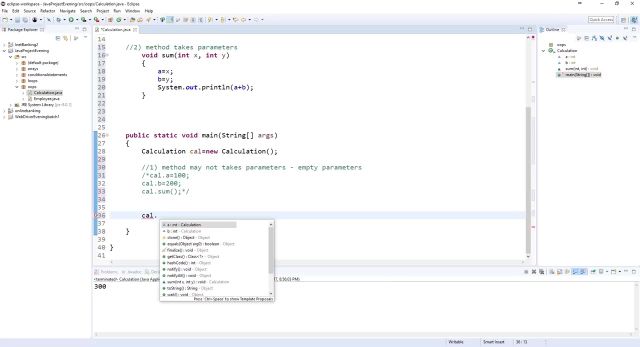 For second one also, we require an object, So cal dot. So this time I don't assign the values to those variables directly like this. Okay, This is not So cal dot, And we'll use Some method directly. Now here I will pass two values. Let us say 100 and 200. 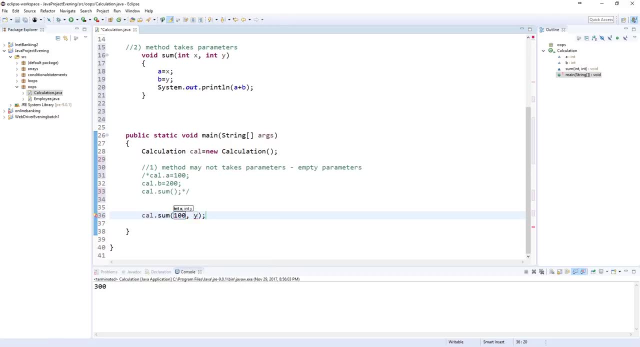 Now what happens is When I call the sum method directly, It will go 100 and 200 will be assigned to the x and y, And x and y assign to the a and b now, And it will perform a plus b operation. 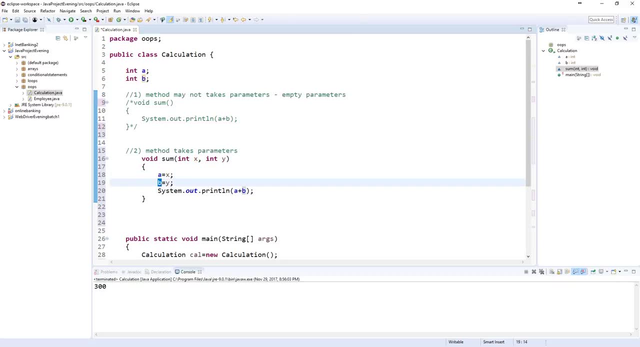 Now See now passing those variables and getting the output. Both are happening at the same time. So now execute this. It will also give the same output. So this is the second. one method takes parameters. This is how we need to write. 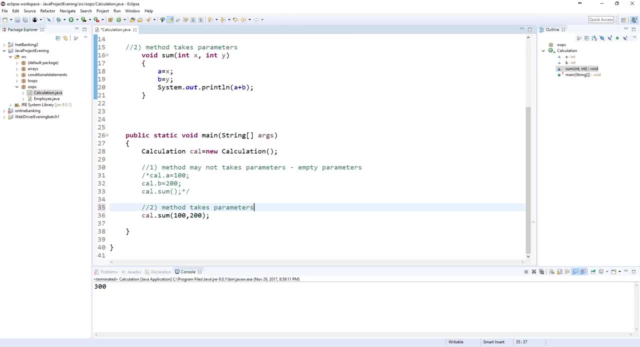 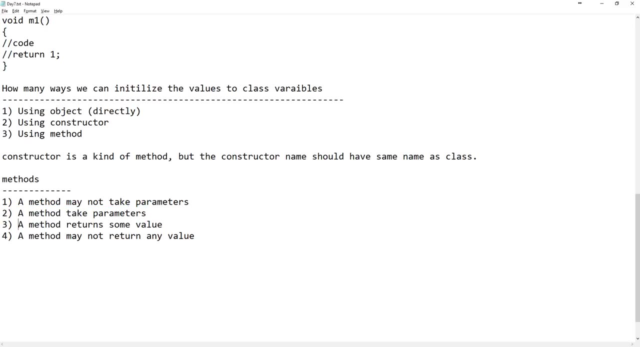 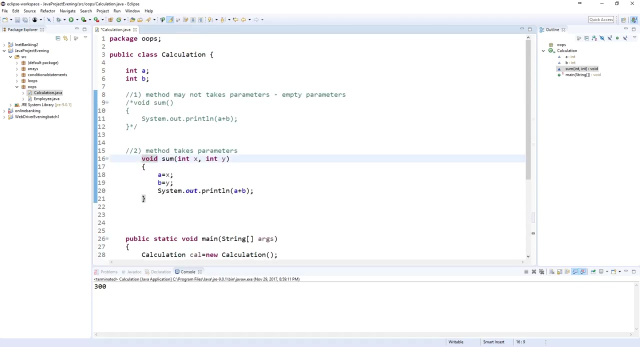 So this is the second. one method takes parameters. The third one method returns some value. Now I will also comment this method. I will write another method. the third point: a method returns some value. Now the same method again. I will write sum and then here, within this method, I will say: 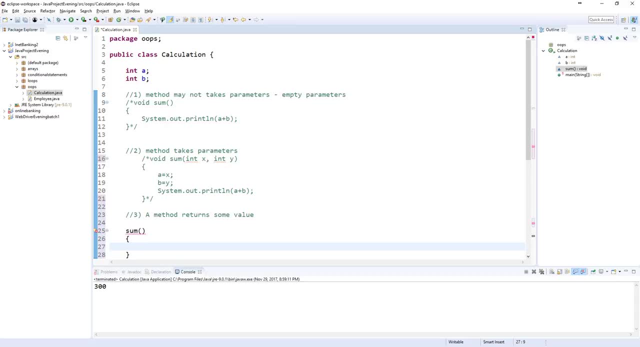 return a plus b. Return a plus b: See this method. So this method, when I call, I am using return statement: a plus b, sum of two numbers. it will do and it will return the result. So the result also should be same type: int type. 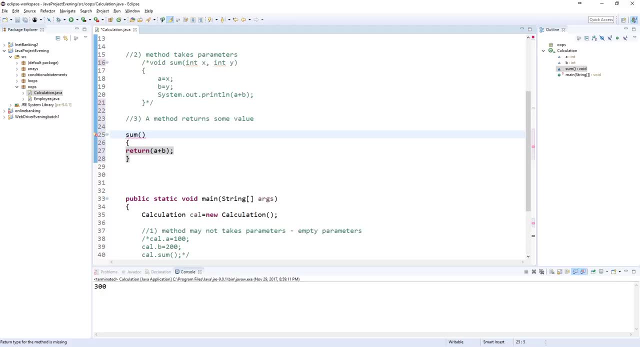 So here we should not specify the void, because this method is returning some type. So this is a method which is returning some value. So now, when I call this sum method, I will comment this also. now the third thing is this one. So this is the third one. 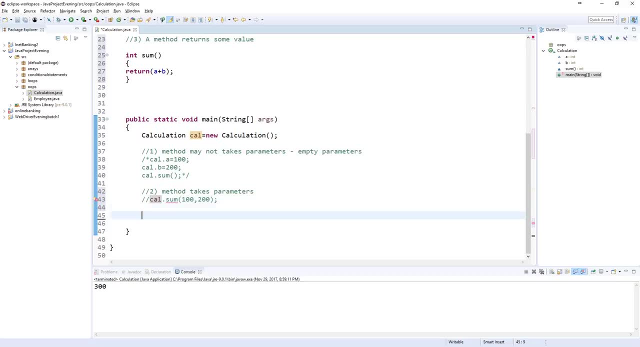 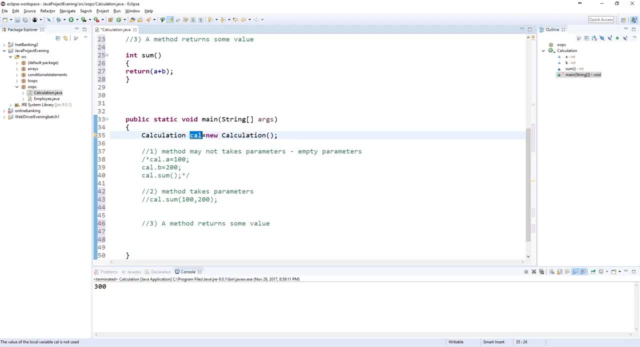 right values. So for that what we can do is we can assign the values by using object itself. Cal dot a is equal to a hundred. cal dot b is equal to hundred. Now values are ready, then I can call this method directly. 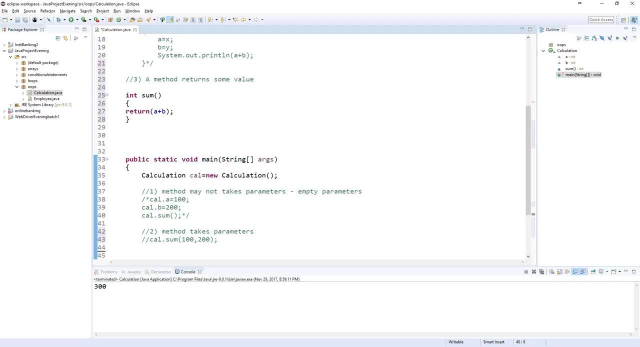 So now cal dot sum, just cal dot sum, nothing. So what happens now? Nothing. A, B are already assigned. Now we have called the sum just calsum. This method is called, It will just return A plus B. It will not print the output. So this method is returning some. 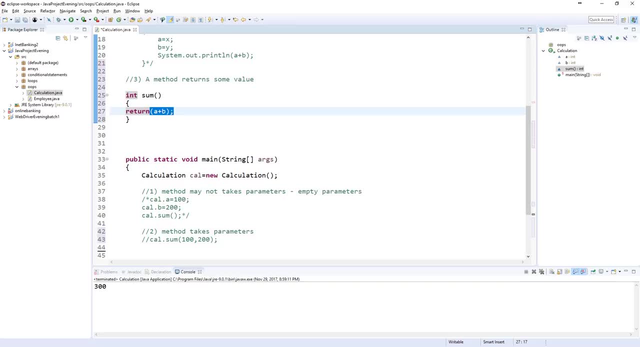 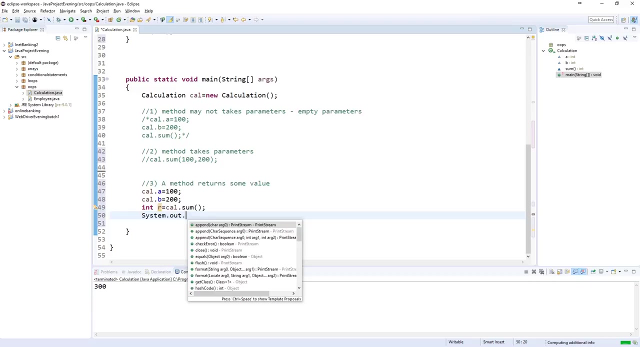 output right. So that output we need to capture into some variable. here, Let us say: int result r equal to calsum. because this method is returning something right: The returned value. we need to hold it in some variable. Now, here we need to print that. So, because that method is, 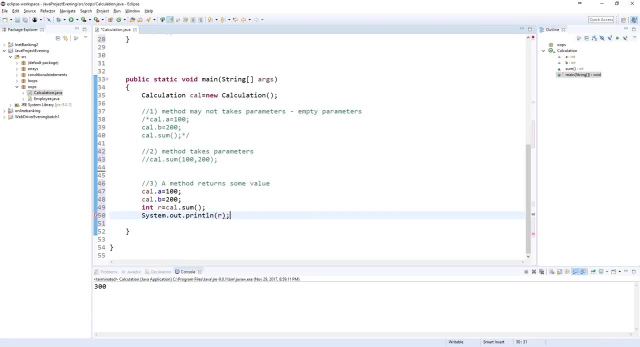 returning some value. that is the reason we need to hold that value in some other variable and then print that value here. Now we execute this, It will give you the same number, because calsum is called. It just returned A plus B Before that itself. 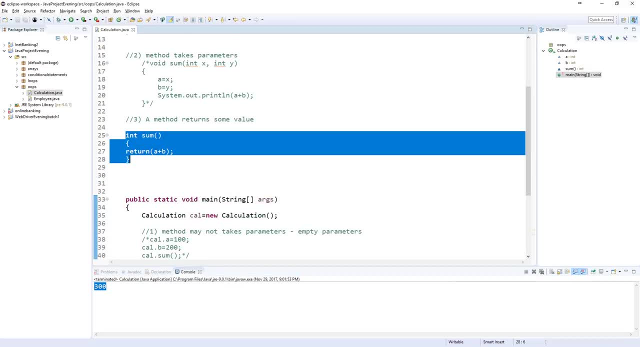 we have a value of A plus B. So we have a value of A plus B. So we have a value of A plus B. Ascend these values. okay, This is the third method. So method returns some value In that. 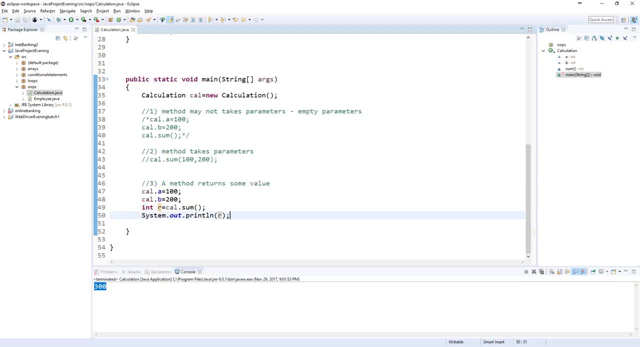 case we need to reuse the return statement. Instead of void, we need to specify int, And here, instead of calling this method, we have to use another variable to hold that return type, and then we need to print that result value. This is the third method, And there is another way. 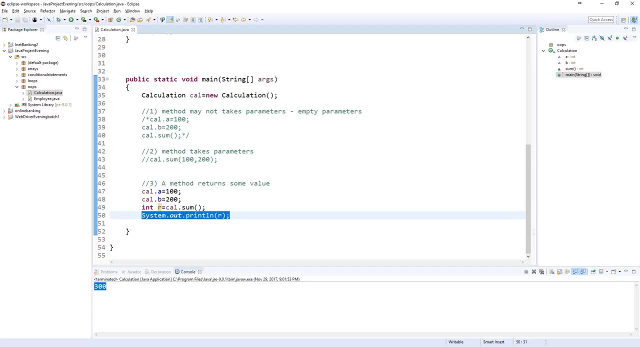 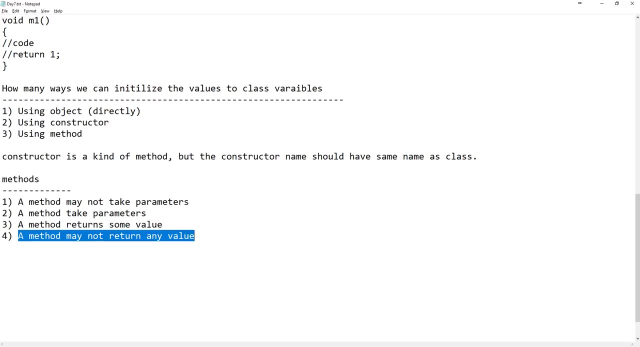 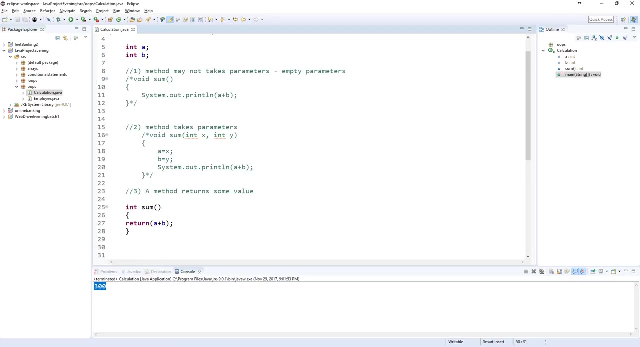 Method may not return any value. Sometimes a method may not return any value. May not return any value means it will print the output directly there itself. okay, So this is an example. The first one is example. It will not return any value means that, basically, is a void. 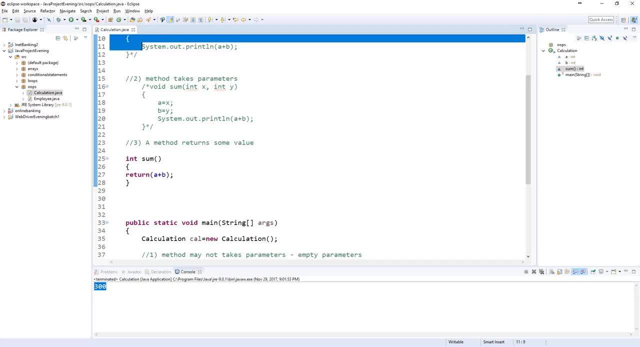 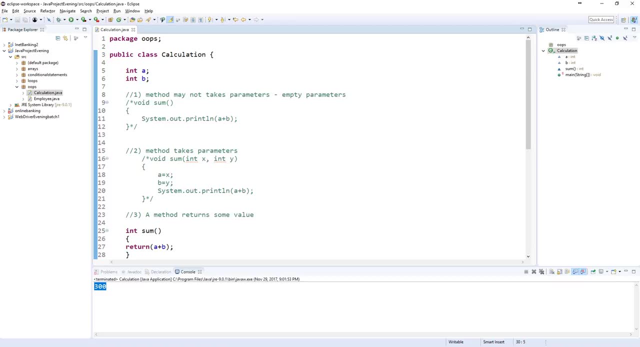 So, for example, the first one itself will come again. So if I say a method may not return any value means there is no return statement, In that case what this will do, It will print the output there itself by using println statement. If you see the first case, a method is there, It is not. returning any value, because face value is not there, So it will not return any value. So here there is nothing. So this way you will add an additional variable for this context. Therefore, you can also use return statement to pack it instead of the product. yes, so that the first 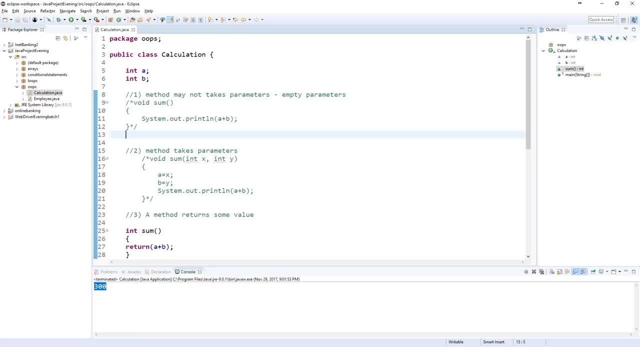 one comes as a房 đây itself. This method is given to the second learning discussion. in the video we are going to go to buildbrowser rendered things. now we have written, We are creating this, these methods, by surgically, indirectly between the first and the end, When in fact 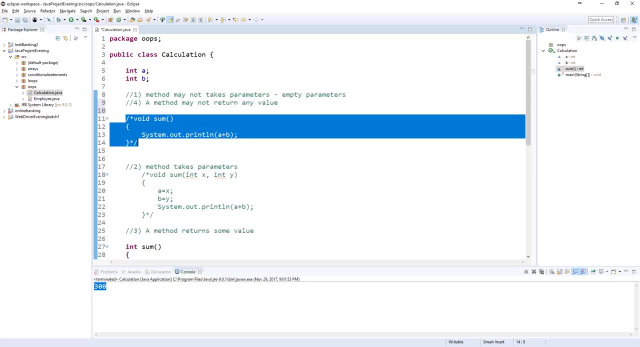 all of the methods are given in. the first was write to get. In fact, if there is any public solution, This component is the one that we are actually going to use. We do not run it, We actually just so. second is: it is taking some parameters but not returning any value. third one is it is not. 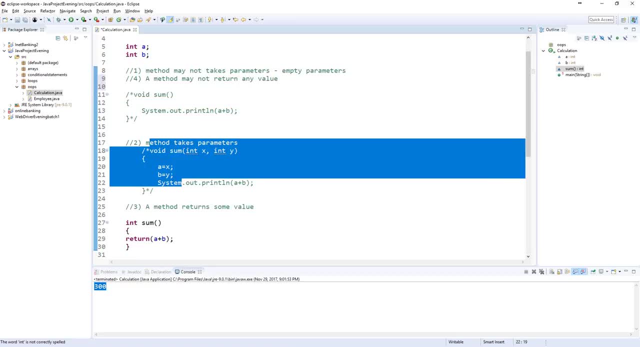 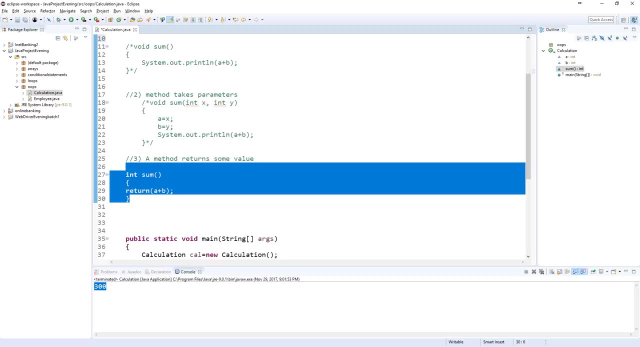 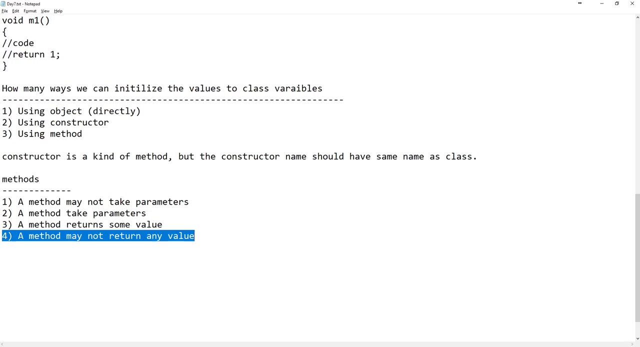 taking any parameters but returning some value. so these are all multiple combinations you can create that is up to your requirement. okay, so, we have learned this concept. a method may not take parameters. sometimes it will take parameters. a method may return some value. sometimes a method may not return some some values. okay so, but if a method returning some value, we have to specify the. 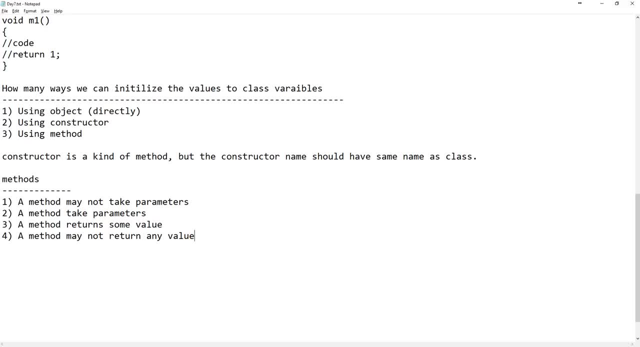 data. one more important thing is i wanted to tell you one difference between constructor and method. so in the previous example i have used one constructor here, right, and this is a method. if i see both of them, it very similar. and what are the differences you can observe here? 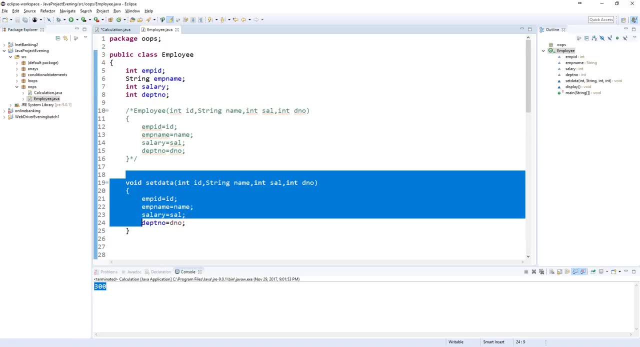 constructor name is same as a class name, but method name can be anything. so this is the one difference you have observed. you can see that the constructor name is same as a class name, but the method name can be anything right other than this. what is up? what is the difference you observed here? for method, we 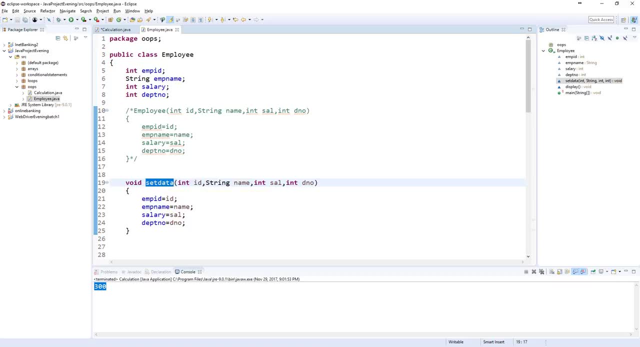 specified as a void, whereas for constructor we haven't specified anything. why? because constructor will never return any value. constructor will always use it for initializing the values, not for writing some logic, not for returning any value. so that's the reason: by default, constructor doesn't return any value, so that we no need to put even void also. 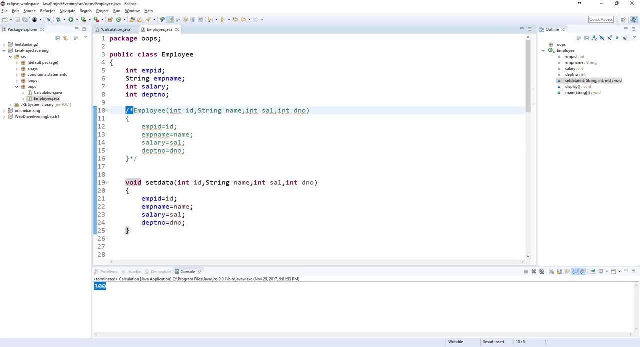 there is a reason for constructor before constructor. i haven't put void statement here, whereas method, if it returns, doesn't return anything. we must specify the void. if i remove the void, it will throw an error. okay, that's the one more difference you can observe between constructor and method. so in the next class we will see in detail what is the constructor, what